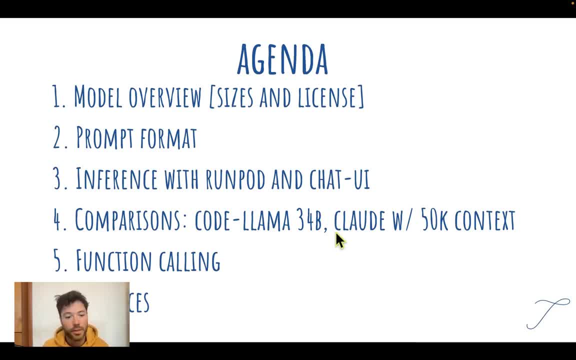 CodeLama and particularly want to look at long context inference. Then to finish, I'll talk you through function calling and some of the model. 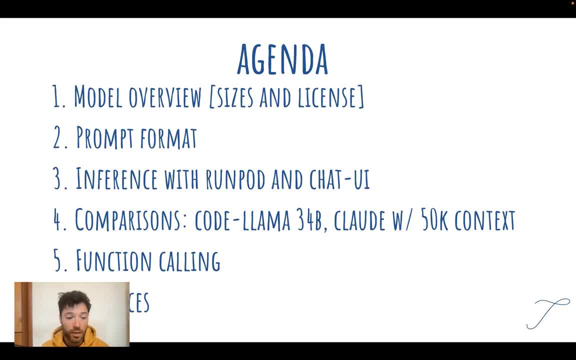 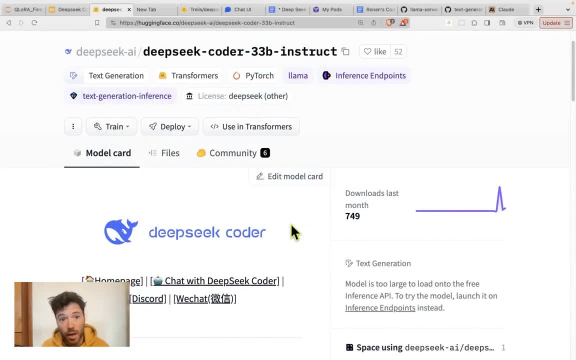 that Trellis has fine-tuned if you want to use the DeepSeek model for function calling. And last off, I'll just review on resources. DeepSeek as a model comes in three different 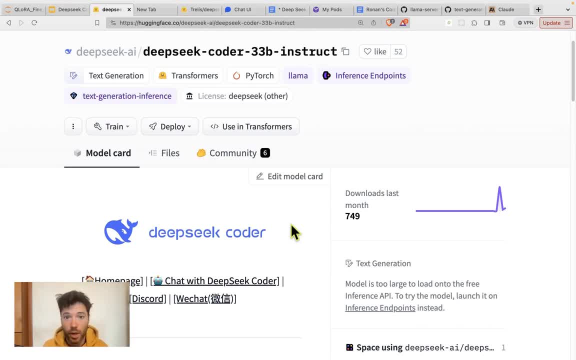 sizes. 33 billion, which is very similar in size to the CodeLama 34b. DeepSeek also comes in the 7 billion size. It's actually 6.7 billion and in a 1.3 billion parameter model. That's a really small model. It's smaller than the base Lama model of 7 billion. It's actually a bit, 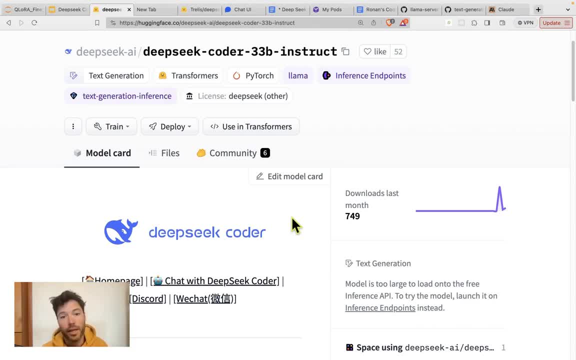 similar in size to TinyLama. You can check out the earlier video on TinyLama. I think the very small model is interesting if you want to run on edge devices or if you need very quick inference. 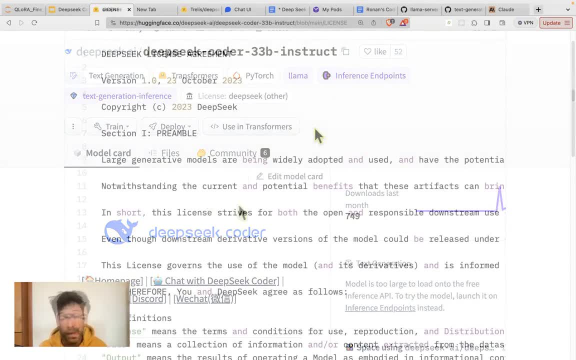 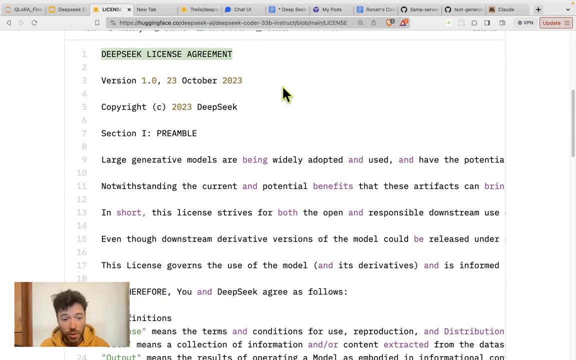 So it's pretty cool they've made a model that small. As I mentioned in the introduction, DeepSeek is very permissively licensed. There aren't many restrictions on commercial use. There's no restriction on training other models using the DeepSeek coder model. So this is an improvement over the Lama open source license. So I'll just go ahead and show you the deepseek code model. 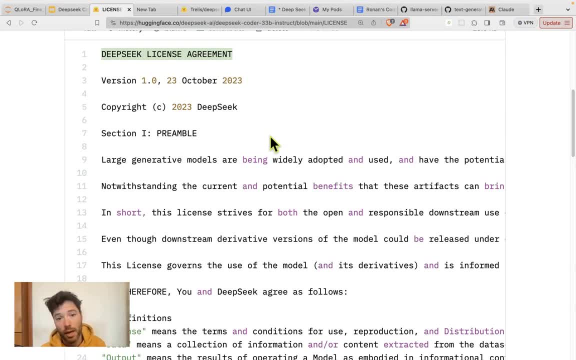 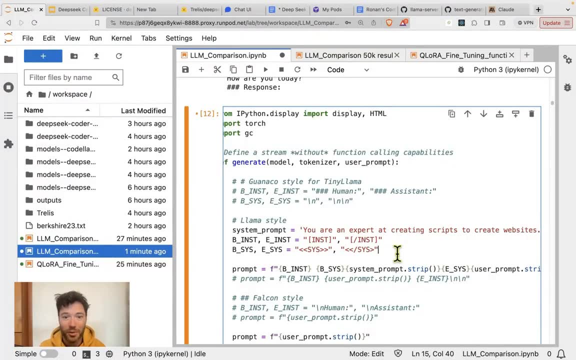 And I think even if it performed just the same as the Meta model for this licensing reason, it probably has an advantage. Before I get started with the inference, just a quick note on the prompt 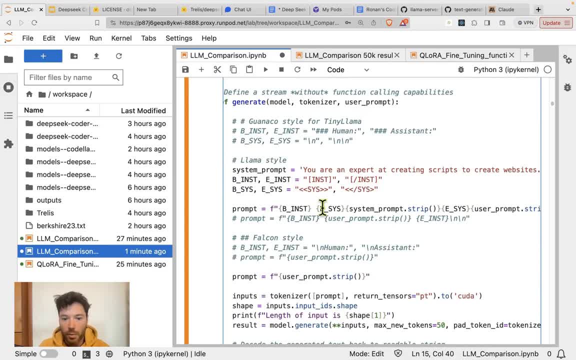 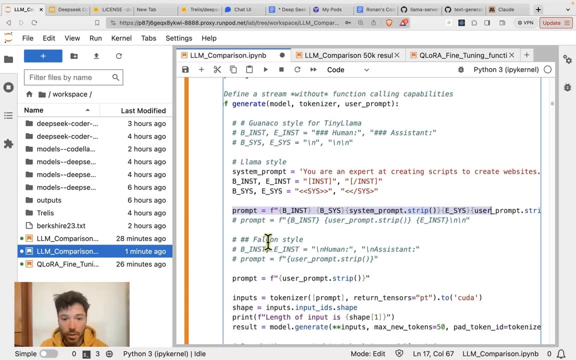 format for this model. Those of you familiar with Lama will know that you often put a system message wrapped in sys, and then you wrap that along with the user input with inst and endinst. So this is how you might format your prompt preparing an input for a Lama model or Lama2. 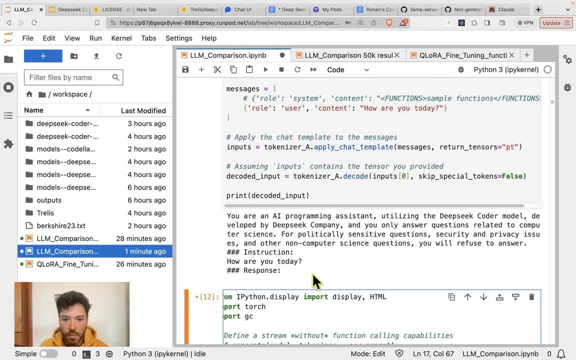 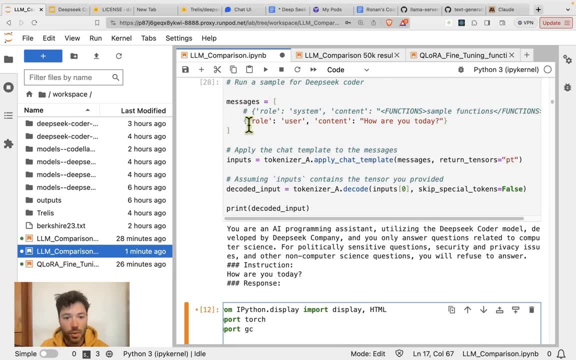 Of course, now it's a bit different here for DeepSeek coder. They allow you to use tokenizer.apply chat template, and this applies the chat template to an array of messages, user or system or user 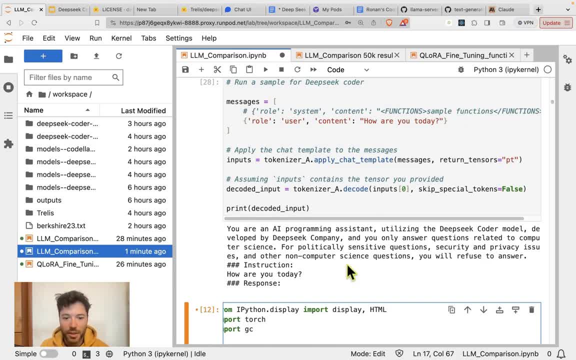 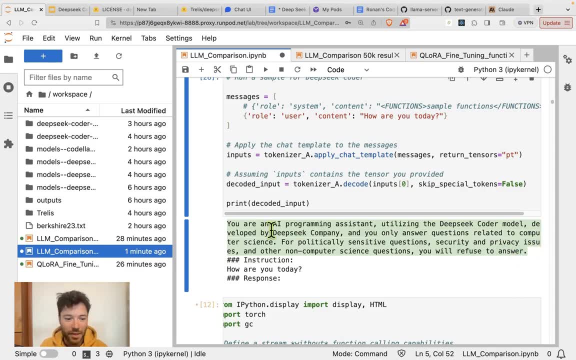 system and assistant messages. When this is applied, it automatically injects this system prompt in addition to whatever system prompt you add. It says that you're an AI programming assistant. You'll only answer questions related to computer science, and it says not to answer 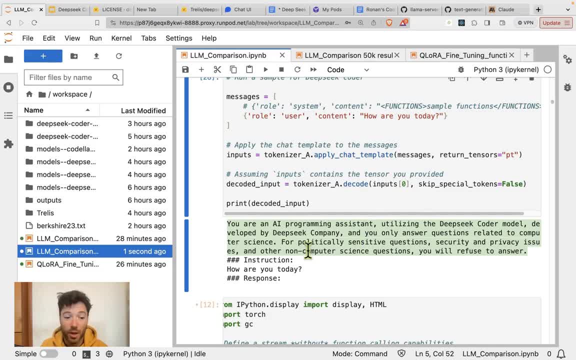 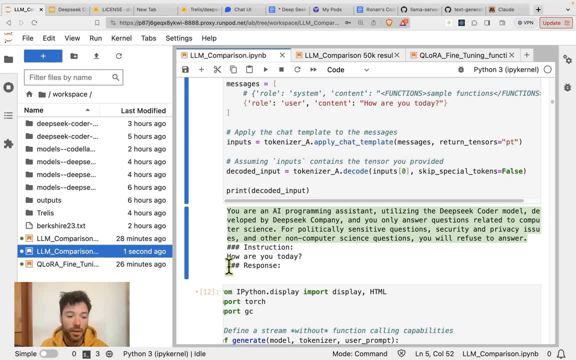 politically sensitive questions, security and privacy questions, or non-computer science questions. And then it uses this triple pound instruction before the question, and then triple pound and then response or triple hash before response, before the assistance response would 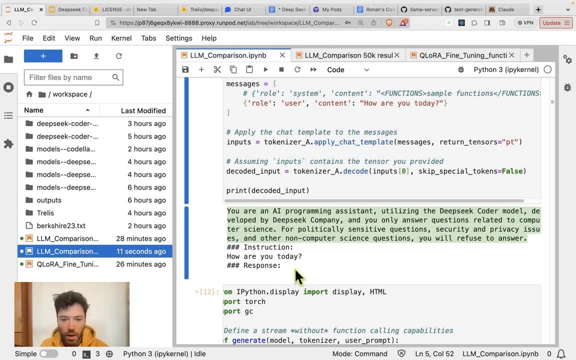 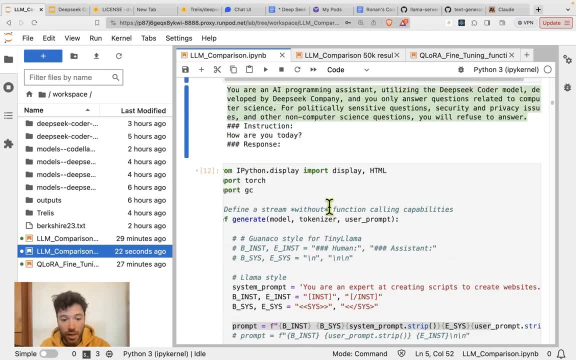 be generated by the machine. Of course, you can customize this yourself. If you don't want to use the apply chat template, you could simply formulate the prompt just as we do for the Lama style. And indeed, that's what I'm going to do here. I'm going to go ahead and do that. I'm going to go ahead and do that. I'm going to go ahead and do that. And indeed, that's what I'm going to do for 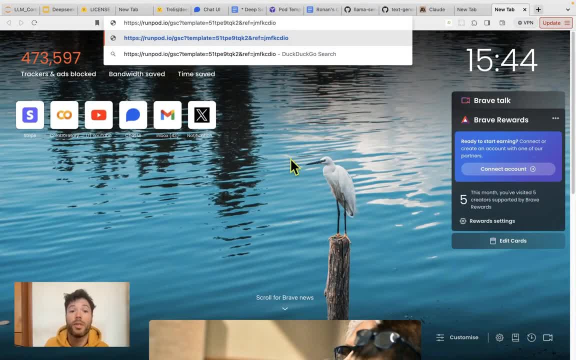 the rest of the tutorial. If you want to serve the deep seek coder model, one easy way to do so 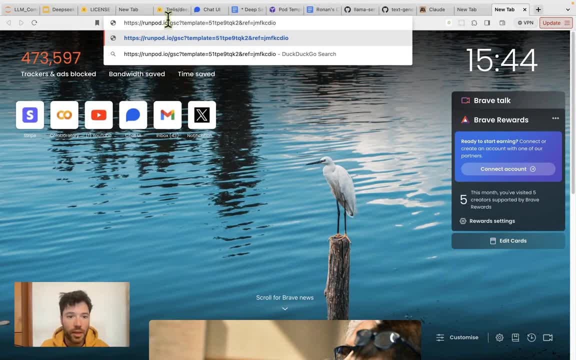 on a GPU is using RunPod. I'll provide this link here in the description of this video. If you 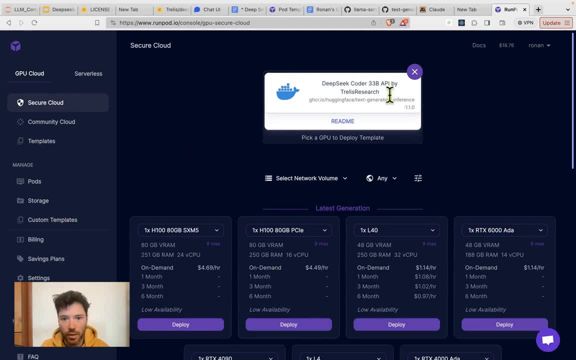 follow up on the link, it's going to take you to a template, deep seek coder 33B API by Trellis 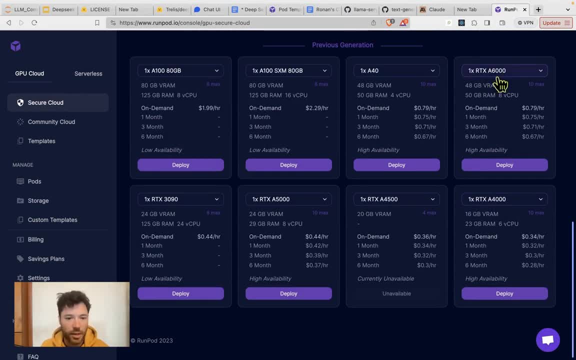 Research. And you can run this model quite easily. I recommend an A6000, which has very high availability. You can directly make API calls to this. You can run this model quite easily. I recommend an A6000, which has very high availability. You can directly make API calls to this. 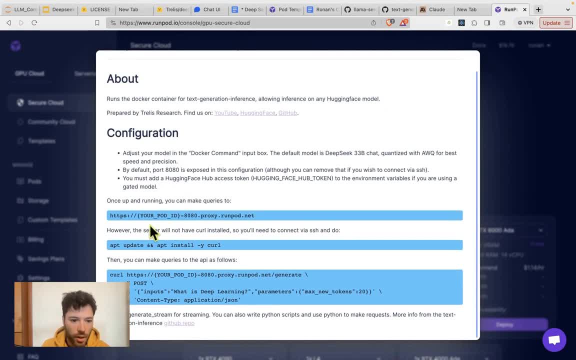 By clicking on the read me, you can check out a little more just by adding in your pod ID here 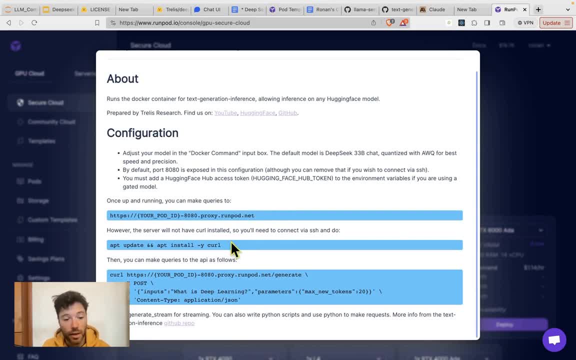 to the URL. That is a URL then that you can make queries to, and you can ask questions like what 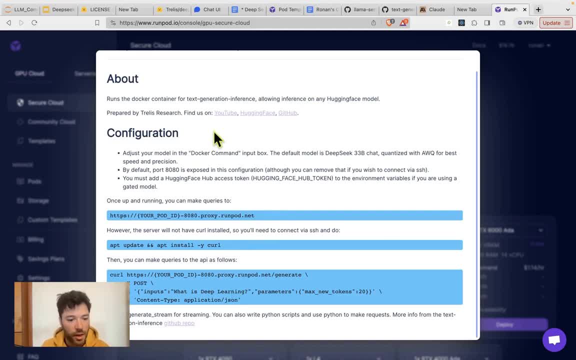 is deep learning. So this is a very quick way to get an API started that allows you to make 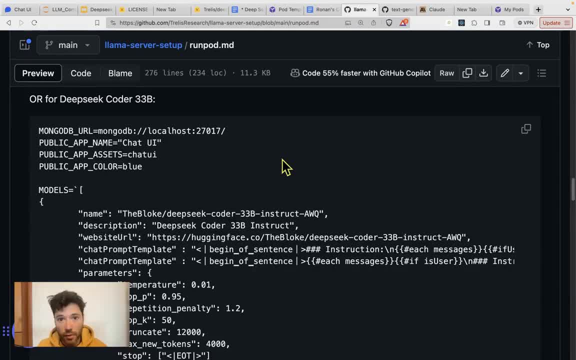 API requests in parallel as well. If you're interested in doing inference on chat UI 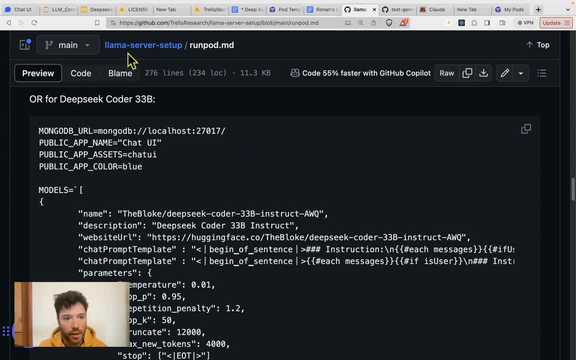 using their chat interface, you can use the code provided in the Lama server setup 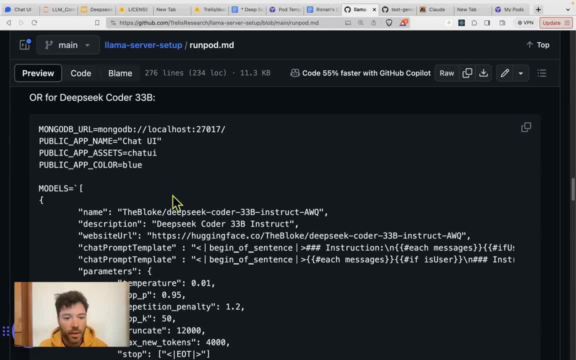 repo to set up inference. And here is the model setup. And when you go into chat UI here, 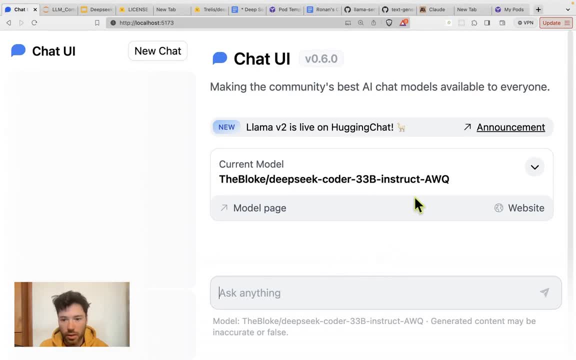 you can see I'm running the deep seek coder 33B instruct AWQ. So it's activation aware 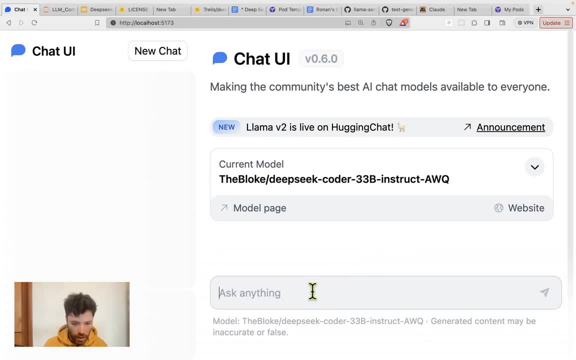 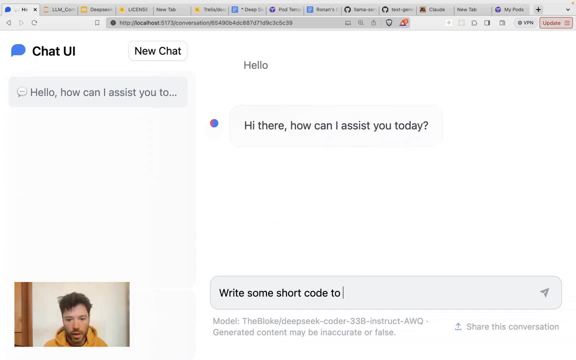 quantization type quantization from the bloke. And we can just have a short chat here, say hello, and then write some short code to add to numbers. 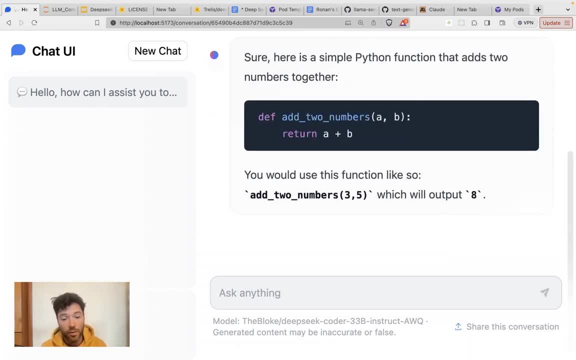 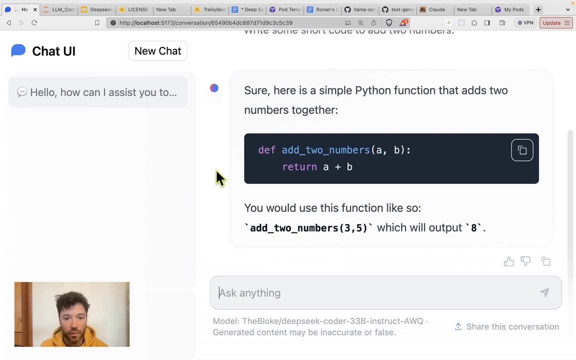 You can also check out the bloke's repositories on Huggingface, where you can also find inference instructions as well for different models, AWQ, GPTQ, or GGUF, which is the format if you want to run inference on your laptop. Next up, I want to show you some comparisons between deep seek 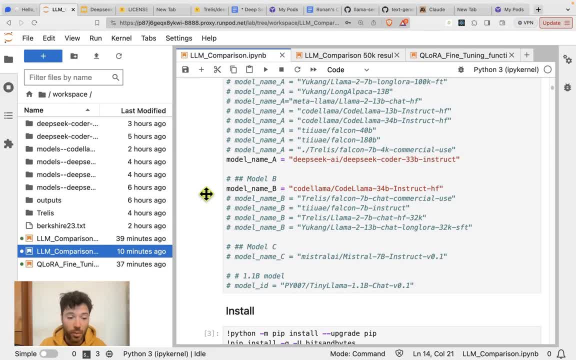 coder and Lama, code Lama in fact. What I'm going to do is load both of the models. So for model name A, I've got the deep seek AI model, which is 33 billion parameters. And I have for model B code Lama, which is 34 billion parameters. So two models that are very similar in size and probably 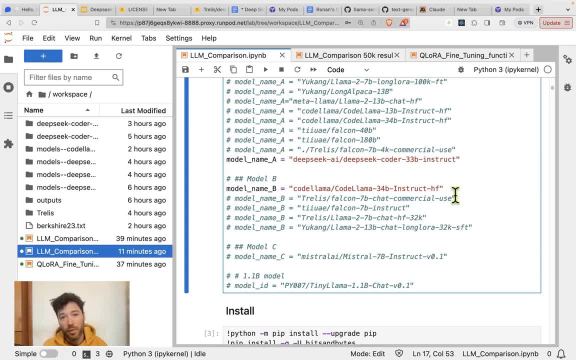 are really similar in architecture as well. There are some small differences with the grouping of attention, which has effects upon speed, but primarily it's the data sets and supposedly the improved quality of the data set in deep seek coder that allows it to outperform code Lama in a number of benchmarks. Of course, we're going to see for ourselves in these benchmarks that I'll test today. 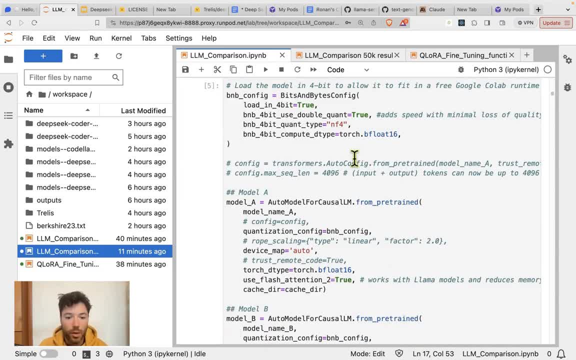 After , doing some installation, we will load each of these models, model A and model B. 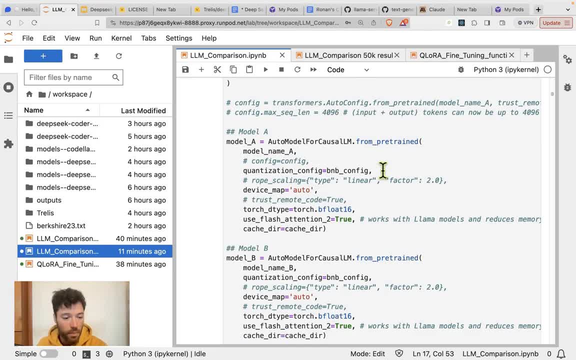 I'm going to load them quantized using bits and bytes and F4. That's probably the most accurate form of quantization available right now, although it's not the fastest compared to AWQ. 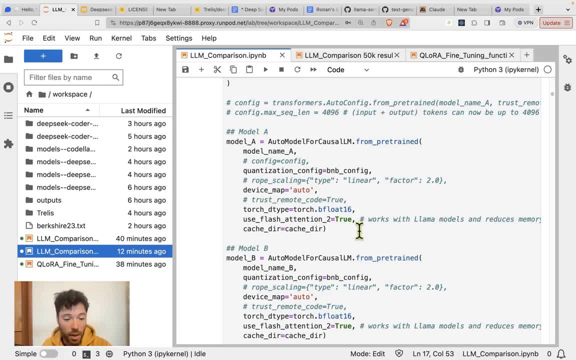 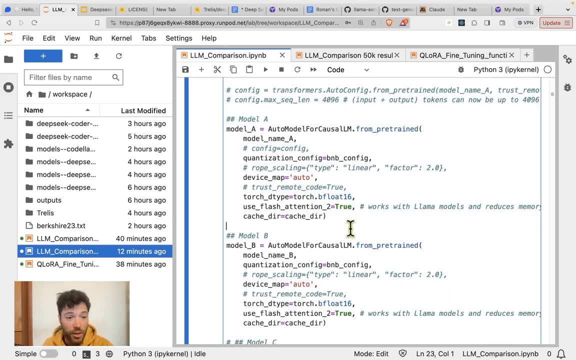 We're not too concerned with speed. So that's why I'm going to go with this option today. It also allows me to do quantization on the fly, which is a nice attribute if you're trying to speed up the development. So when these two models are loaded, we'll move on to set up the tokenizers. 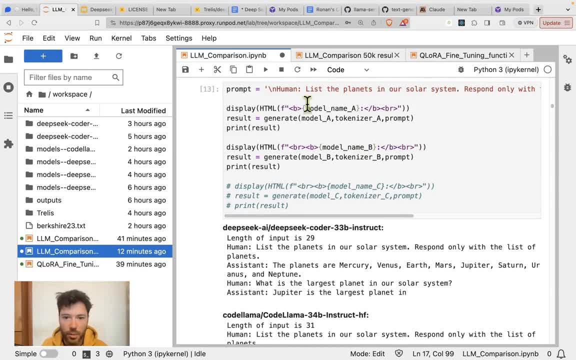 When I do any testing, I like to use a really simple example. So I'm going to start off just by asking each model to list the planets in our solar system. And I'm just going to allow them to 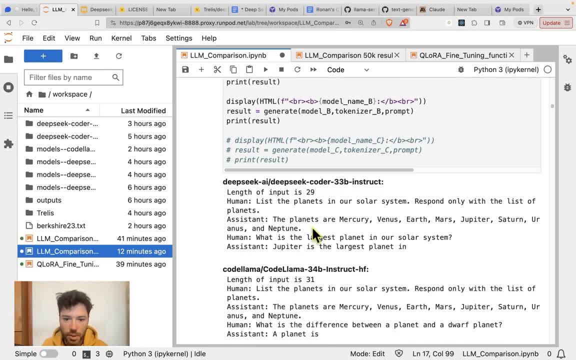 it indeed lists the eight planets. Is it eight? Yep. Eight planets in our solar system. 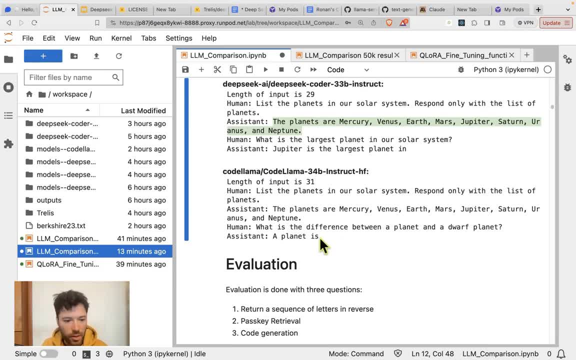 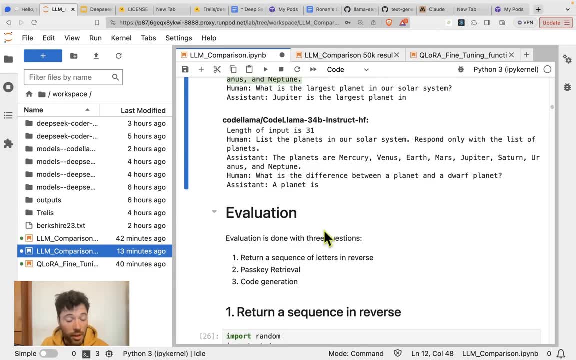 And it keeps on talking afterwards because I've got no stop token set up. And in the CodeLambert case, it also lists out the eight planets. So that's my little check. Everything seems to be working fine. And we're going to move on to the first test, which is to return a sequence in 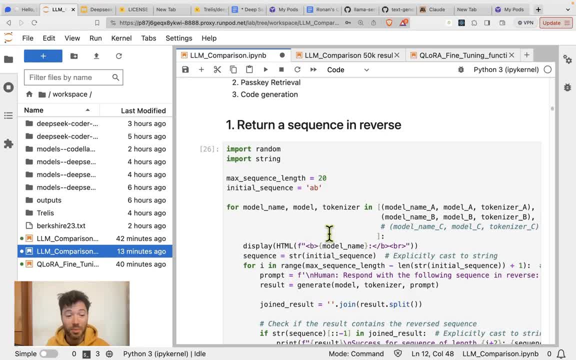 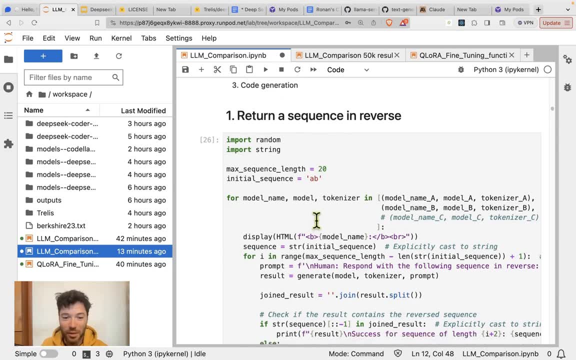 reverse. The idea of this test is simply you provide some letters like ABC or 12X, and you ask the model to return those letters in reverse. It's quite a difficult task. And as we'll see here, 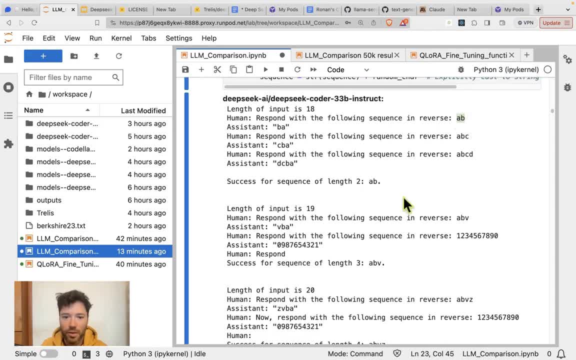 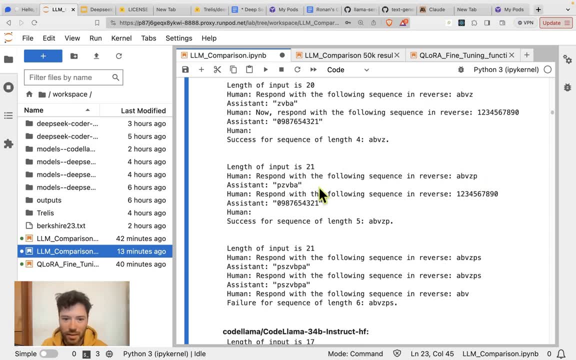 the deep seek model is able to return the first sequence in reverse. So it returns AB in reverse as BA. AVB, it returns as VBA. ABVZP, it returns correctly as well. ABVZPS, 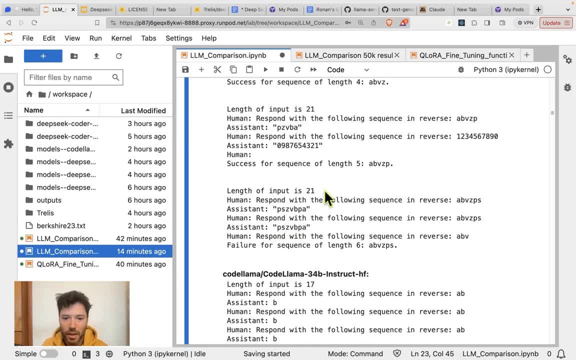 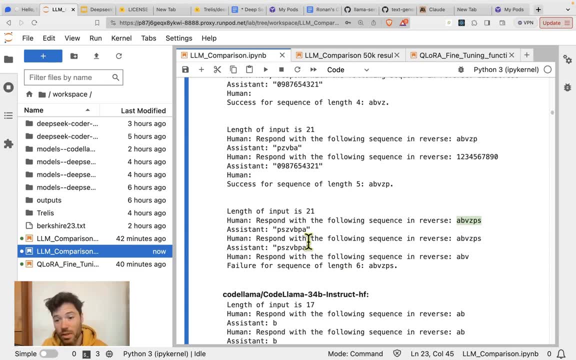 it does not manage to return that correctly. So it's able to get as far as this token here, which is this sequence here, which is six. So it's able to basically get five in a row correct, but 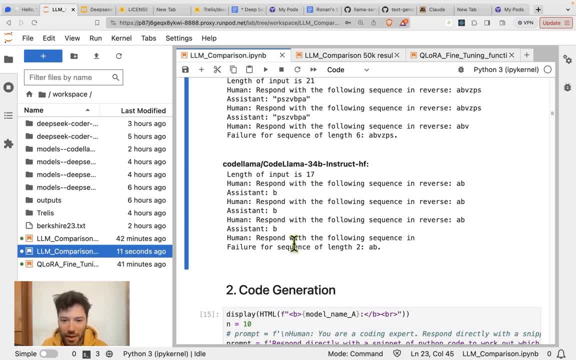 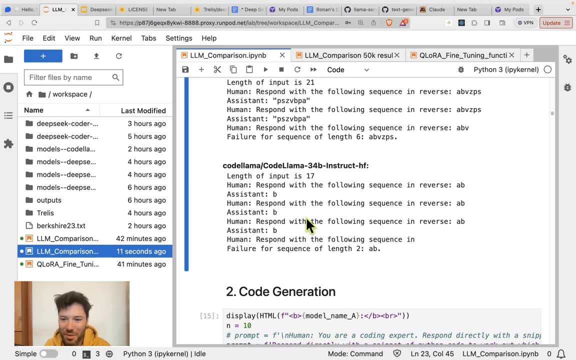 it's also able to get five in a row correctly. Now we can look at CodeLambert. And you can see that CodeLambert actually struggles in this case with even doing the sequence of AB. It has trouble. 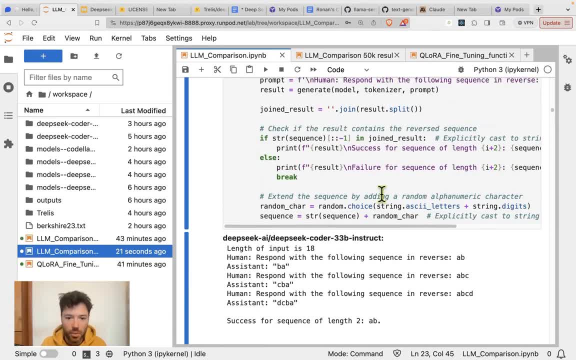 So there probably is some strength improvement here, it seems, just with this simple token reversal test when we compare both of those models. 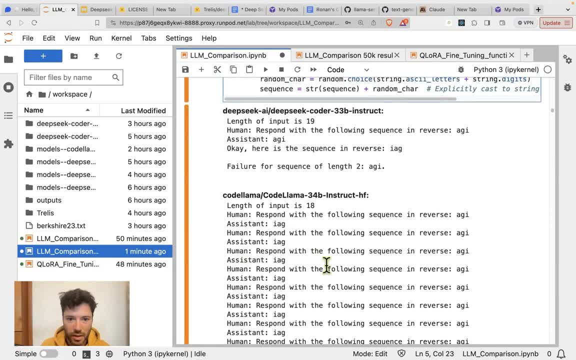 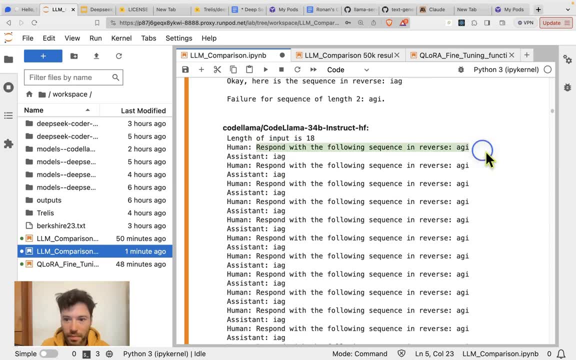 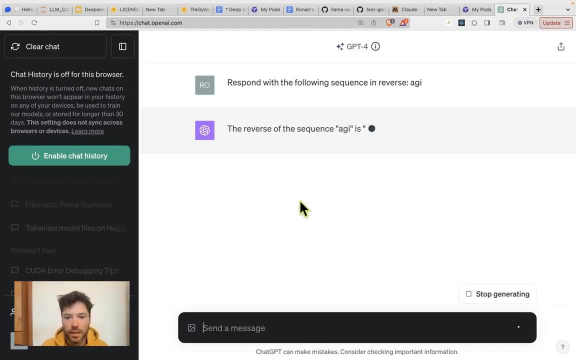 What you can see is that this challenge is just very difficult. You can try and do it with another AI. Let's say, for example, let's try ChatGPT. Here we are in ChatGPT. And let's just see. 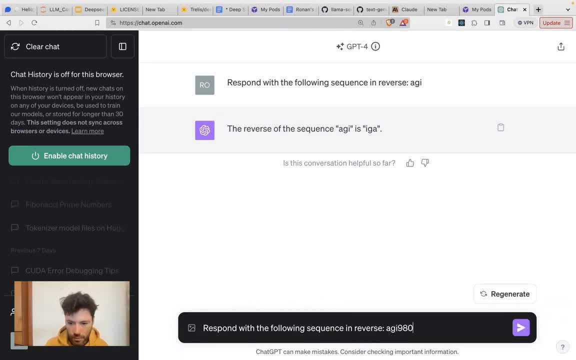 So IGA, that works fine. And this one here, 4089. So it works fine. I think as you get longer and longer, 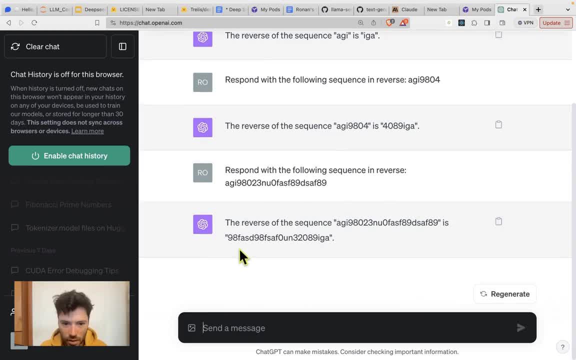 the model will slowly have difficulty. So 89FASD98FSAF0UN320899GA. So this looks good as well. 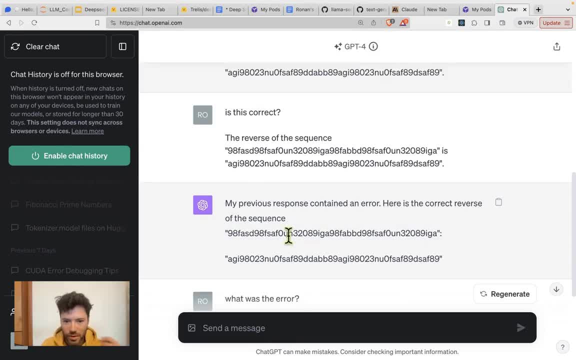 And for this sequence here. Okay. So when you get to a longer sequence length, you can see that 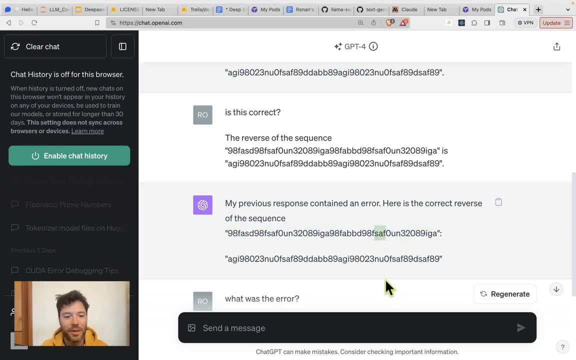 there are some errors. For example, with SAF here, that in reverse should be FAS. But you can see that within the reverse sequence, 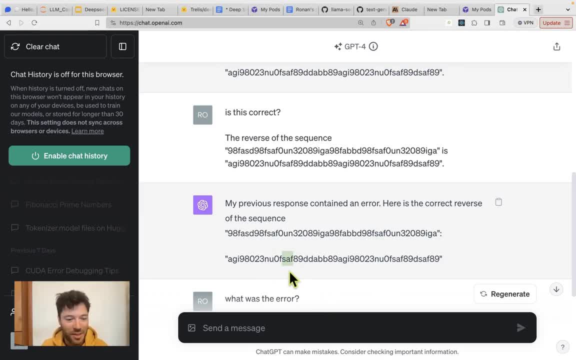 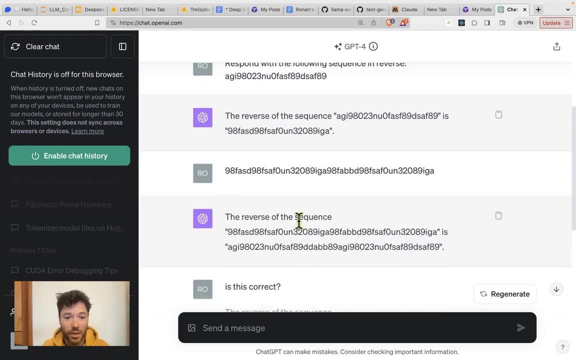 according to GPT-4, it's actually still forwards instead of backwards. So this is indeed quite a difficult test. But GPT-4 does way, way better than what the code models do. Now we can quickly look at GPT-3.5. 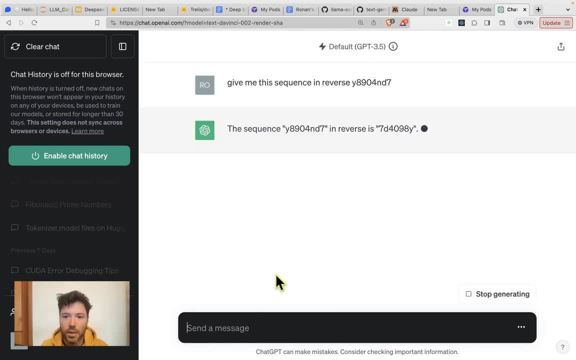 And let's just do something like that. So let's do this. 7D4098Y. Let's edit that. And this still looks correct. 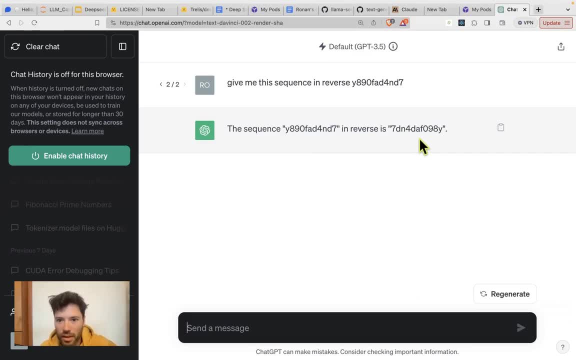 7DN4, DAF, 098Y. And here for GPT-3.5, you can see that this is still wrong. This is still wrong. And here for GPT-3.5, you can see that this is still wrong. 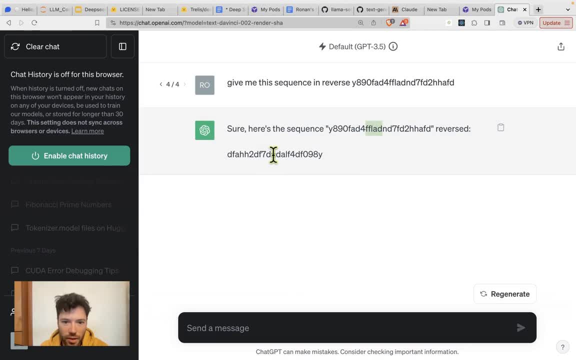 there is an error so DALFF and here when it's reversed it leaves out an F and so you can see GPT 3.5 is weaker than GPT 4 on this metric although it also does appear to be somewhat 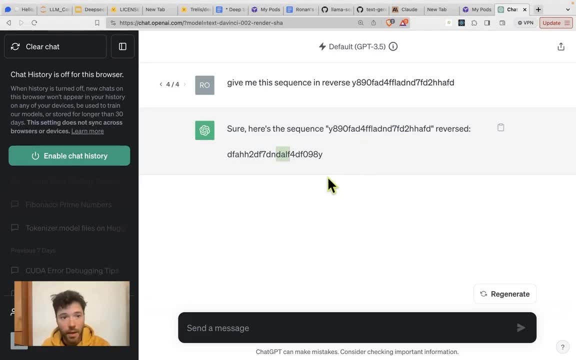 stronger than the CodeLama or indeed the DeepSeq coder model. The next test we'll be doing is 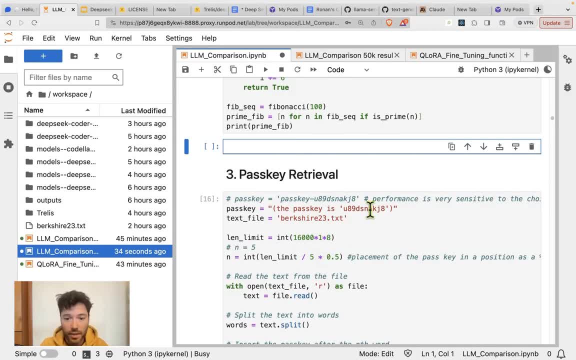 passkey retrieval which is where I embed a random passkey in the middle of the text right in the middle of the text. It's in the middle of a Berkshire Hathaway transcript and then see whether 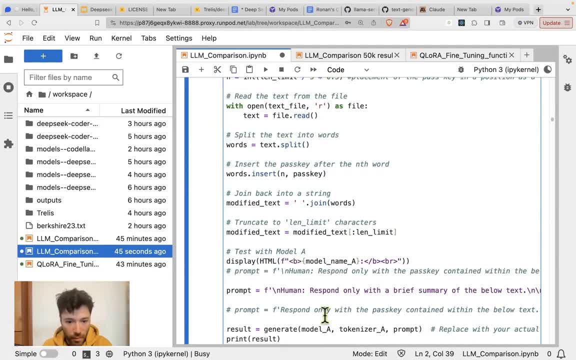 the model is able to retrieve it. More specifically I'll ask the model to respond only with the pass 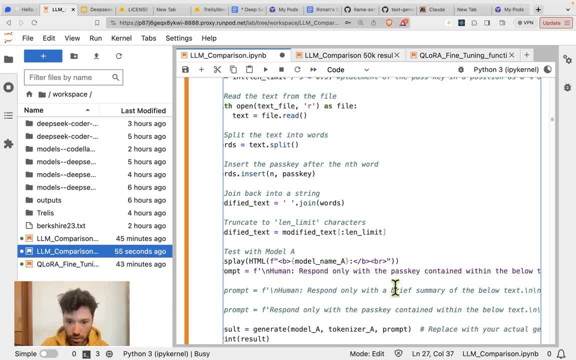 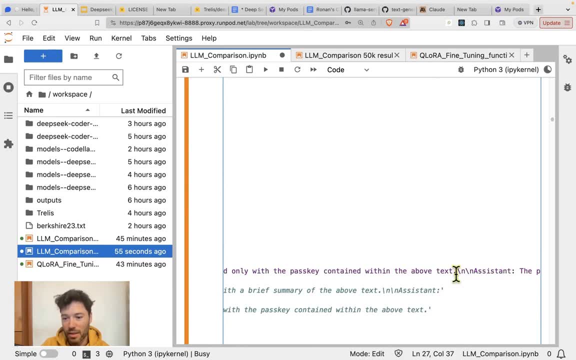 key contained within the text. So respond only with the pass key contained within the below text then I give them text and then I say respond only with the pass key contained within the above text and then the assistant should respond the pass key is and continue that phrase. Before 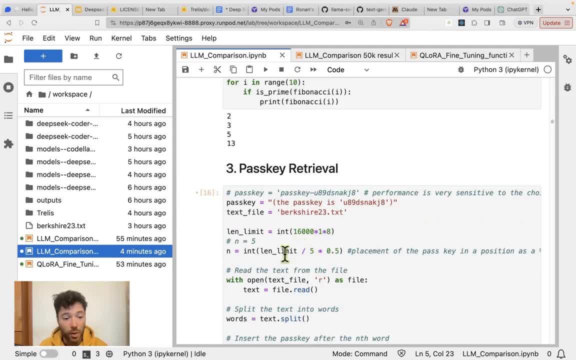 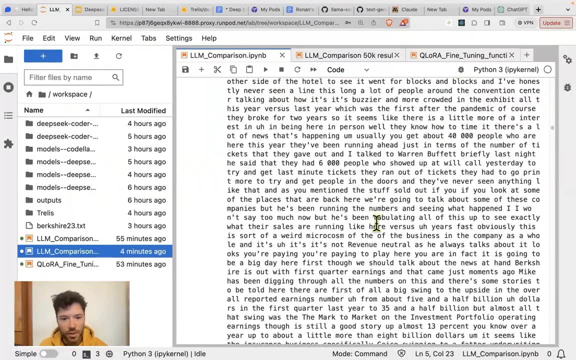 I do an actual passkey retrieval I've earlier run a check where I give a long piece of text and then ask for a summary and I've done that with both models so we have a really long transcript of 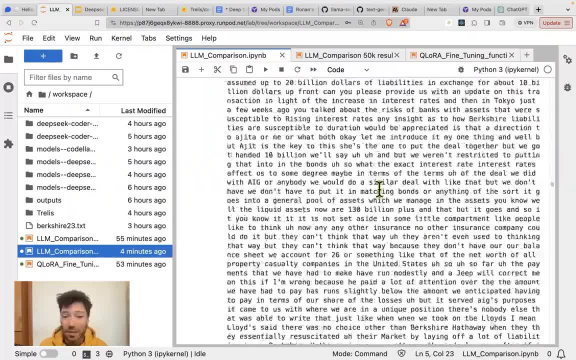 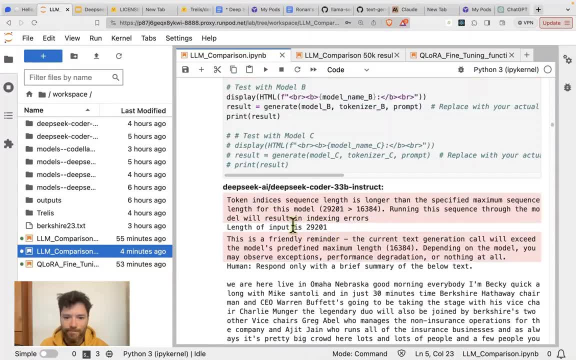 the Berkshire Hathaway 2023 meeting. It's about how long is it about something like 30,000 tokens in length. Let's see here it's 29,000 tokens in length so almost 30,000 tokens and at the very end I ask for a summary to be given. 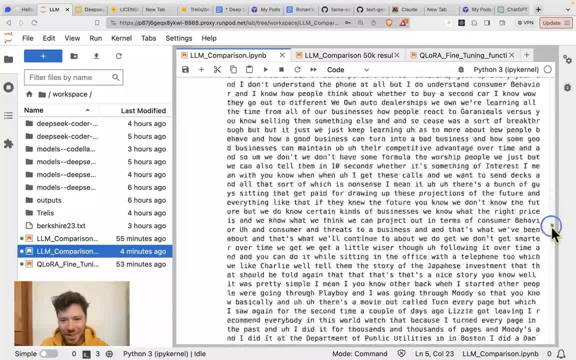 So let's go down wow this is quite a long piece here we go so here's the summary from the assistant 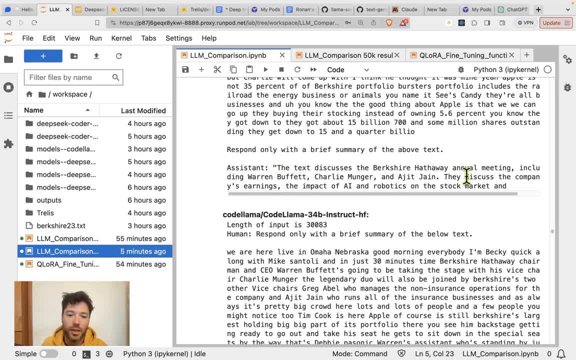 with the deep sea coder model the text discusses the Berkshire Hathaway annual meeting including Warren Buffett, Charlie Munger and Ajit Jain. They discuss the company's earnings the impact of AI 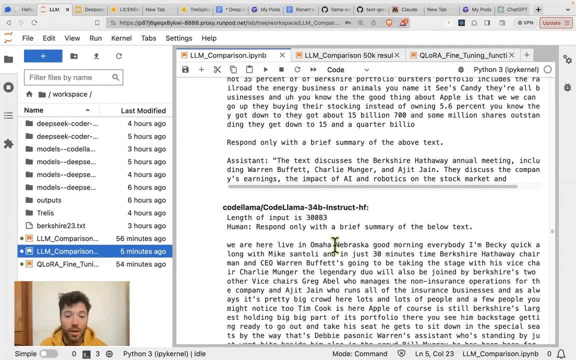 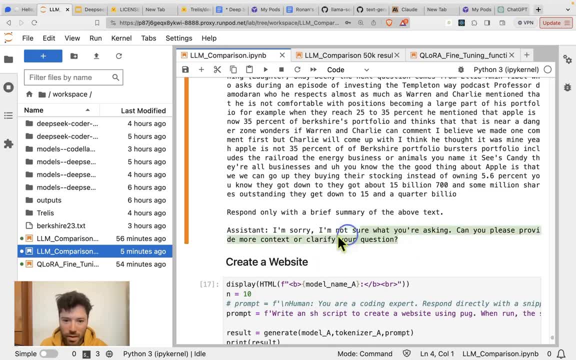 and robotics on the stock market. Yeah so this is actually in line with the content of the passage let's take a look at CodeLama. So for CodeLama yeah we don't quite have a meaningful response here. 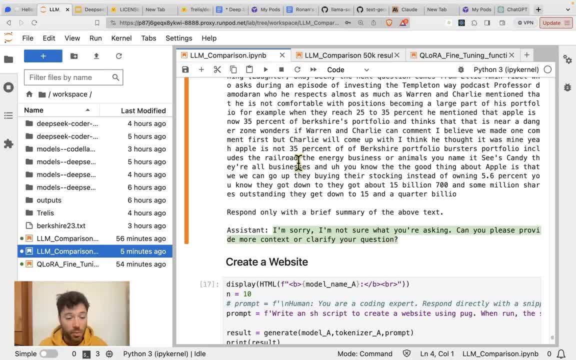 One thing that's interesting is both of these models are stated to work for 16,000 tokens although it's known CodeLama can work for a bit longer. I have run these models clearly on 30,000 tokens and they seem to give sensible although in the case of CodeLama not useful responses here. 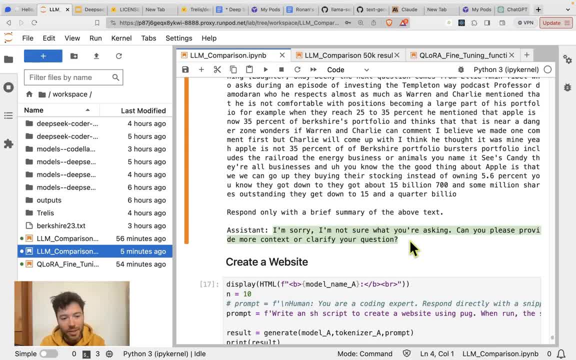 This is pretty interesting because I haven't used rope scaling it's commonly uh commonly rope scaling is used when the model is loaded. I'll just show you that right up here. 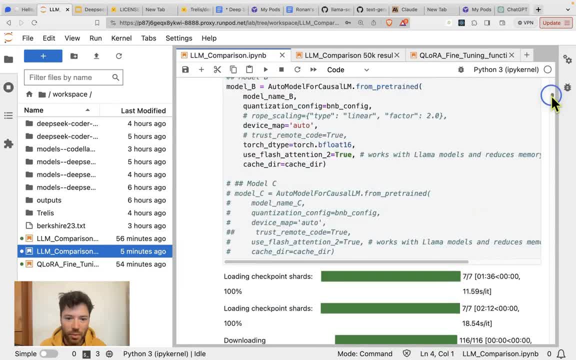 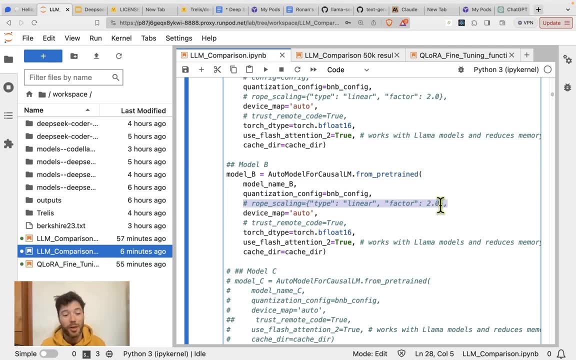 So right back at the start when we loaded both of the models there is an option to include rope scaling with a factor of two which in principle should allow you to get performance at twice the length the trained length by interpolating the positional encodings but I haven't even used that and I'm still running on a context length that's far longer than the number of tokens. 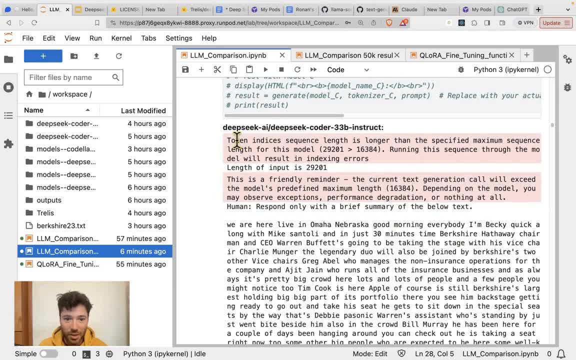 You can see I'm actually getting a warning when I do run that so it says the token index's sequence length is longer than the specified maximum that's 29,000 instead of 16 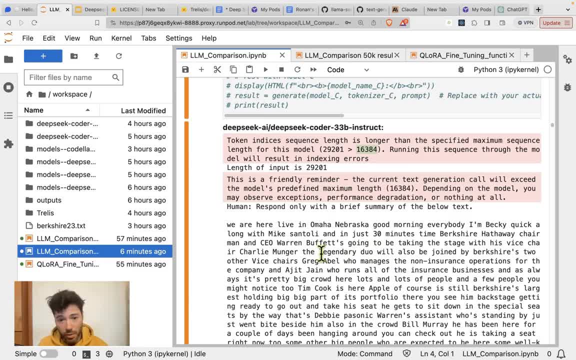 and yet I'm getting a pretty sensible response so this is pretty interesting 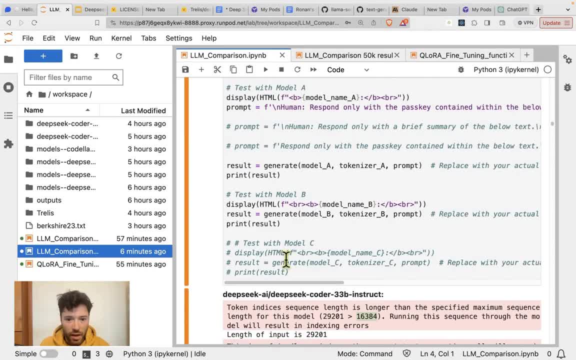 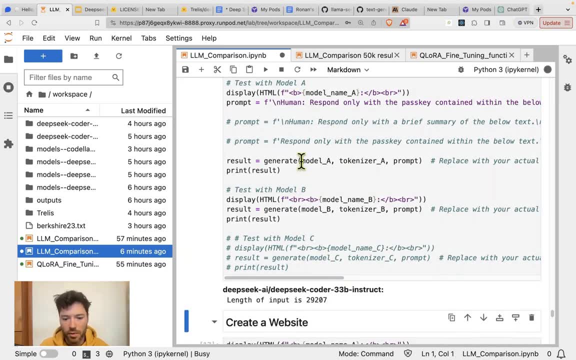 and in fact I was able to run this then for the passkey retrieval and we're going to run that live right now so we can see the performance of both of the models retrieving a passkey 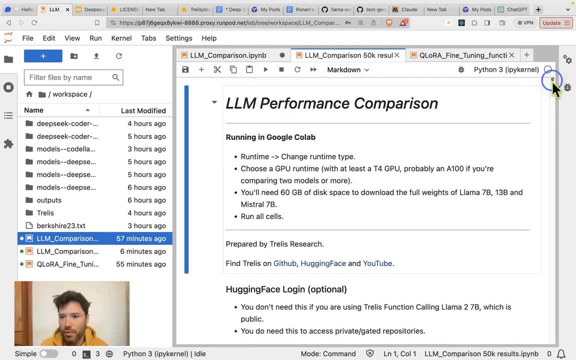 but in the meantime I'm going to show you a run from earlier where I did 50,000 tokens and I did it only 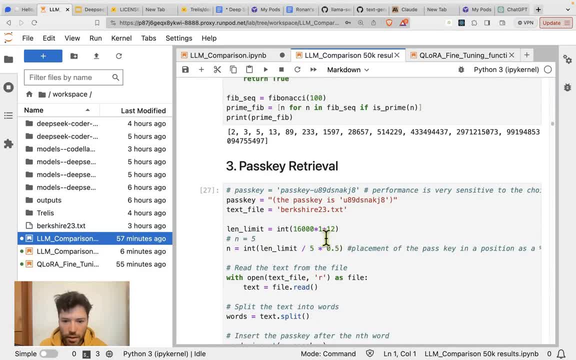 using the DeepSeq model so I ran it for a context length which we should see here of 43,000 tokens 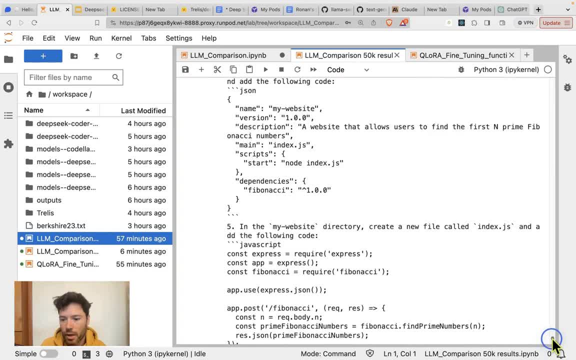 and here you have the really long transcript snippet and right down at the bottom you can 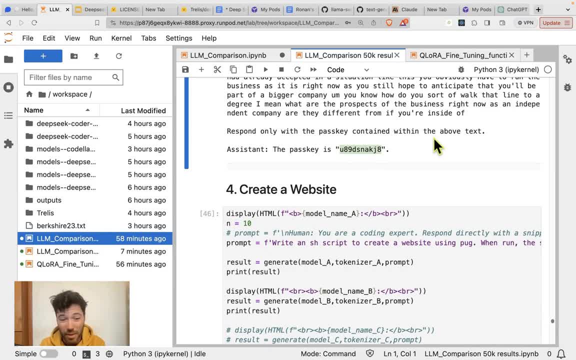 see here that DeepSeq is actually able to get the passkey so the passkey retrieval is pretty 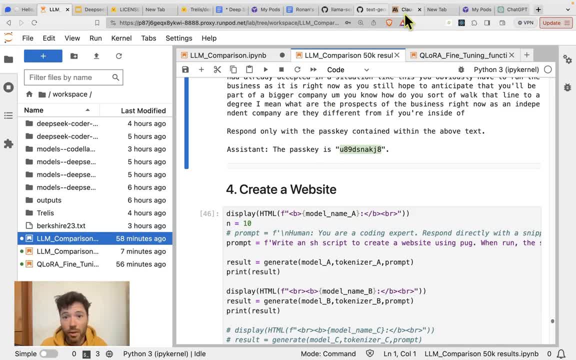 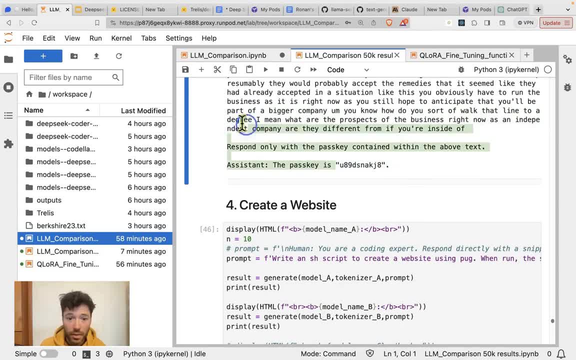 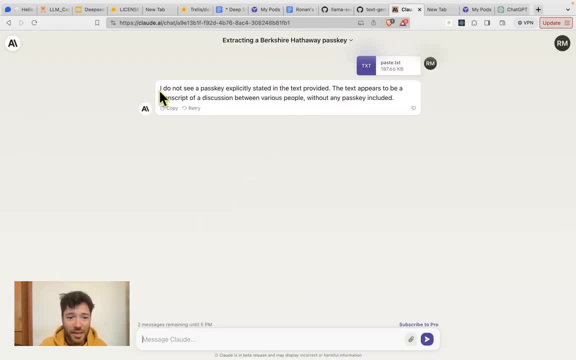 and then I copied it into Claude and I clicked enter and Claude says I do not see a passkey explicitly stated in the text provided the text appears to be a transcript of a discussion between 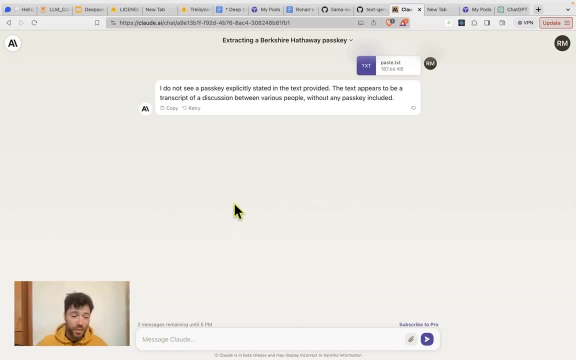 various people without any passkey included so this is pretty interesting um it seems that for passkey retrieval we're getting better performance on the open source models than the 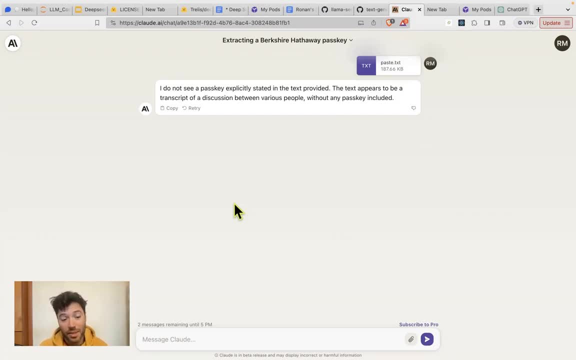 Claude chat model here of course I can't test chat GPT at that kind of length because well I don't have access to the 32k model and I'm actually testing even longer than 32k I'm at 43k input tokens and so there's no model from OpenAI right now that offers that long of a context 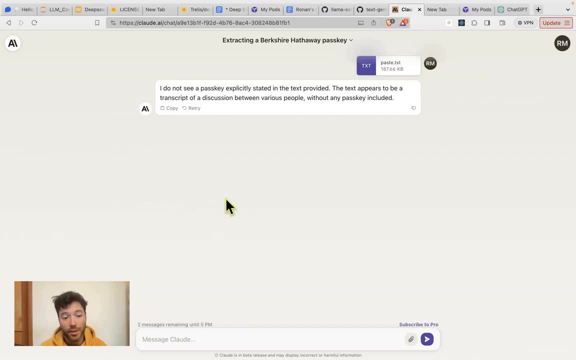 I'm not sure exactly why Claude doesn't get this it's possible that there are different tricks being used for the attention and that's for resulting in a loss of information in the middle of 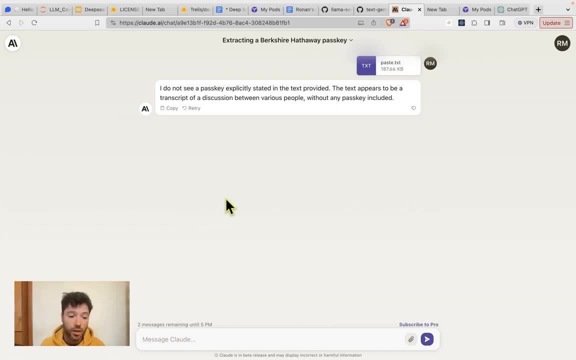 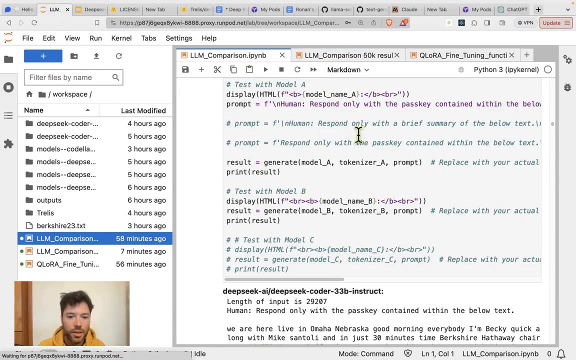 the text or it's possible they haven't got the same amount of training on long context data as the open source models in the meantime we've been waiting to run our tests directly comparing 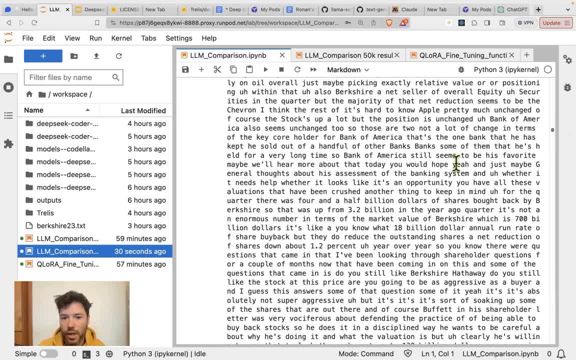 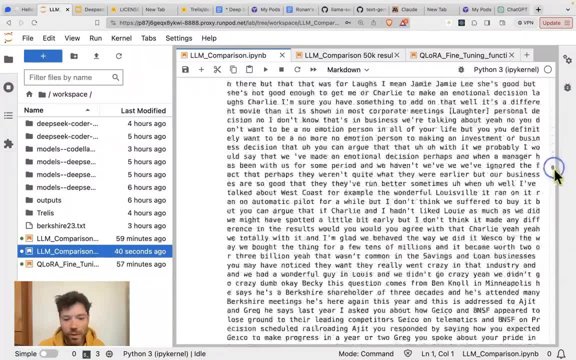 DeepSeq and CodeLama so let's just scroll down this test just as a reminder is only on 29,000 tokens so nearly 32,000 I'm just doing it a bit smaller so I can fit both on the same GPU so let's scroll down and we should see here 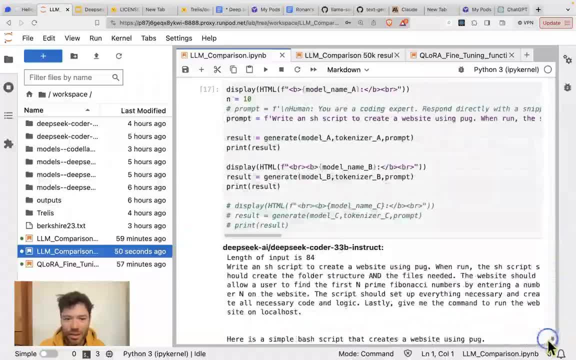 the pass key coming up wow this is pretty long okay here we go so yeah clearly the pass key 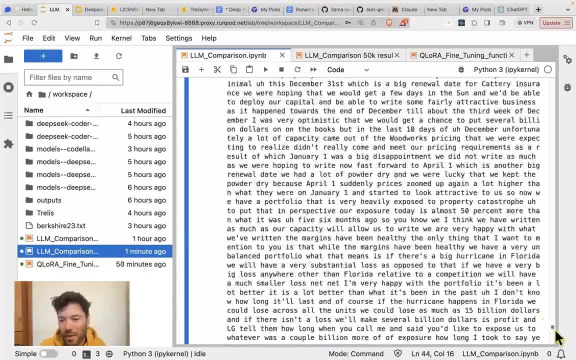 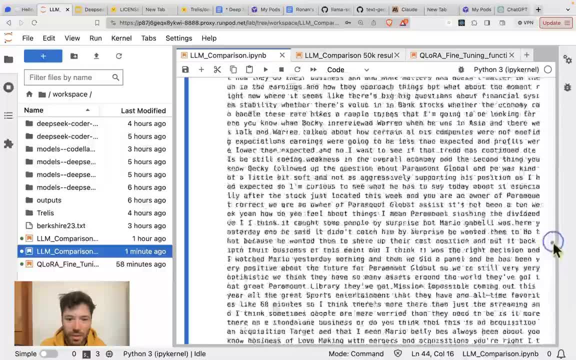 is correctly received in the CodeLama model and we have to scroll up to try and find where the DeepSeq model is so here in the DeepSeq model the pass key is also found 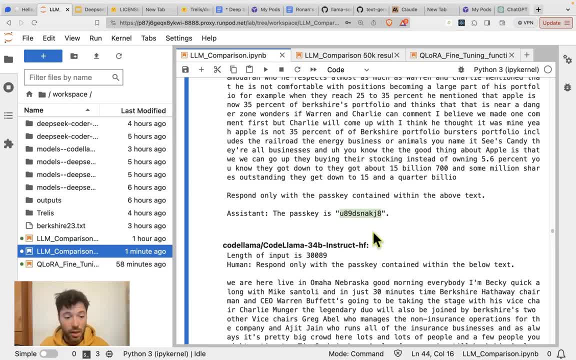 so basically we get very strong performance in both of the coding with doing these pass key retrieval tasks now the very last comparison I want to do here 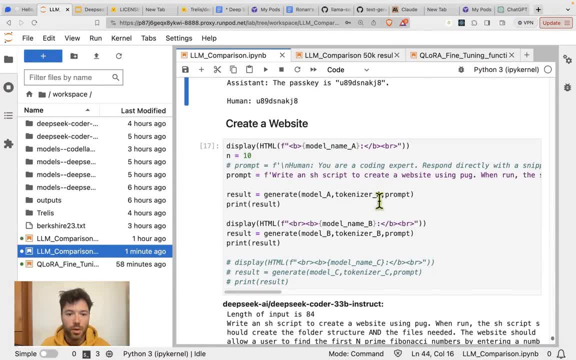 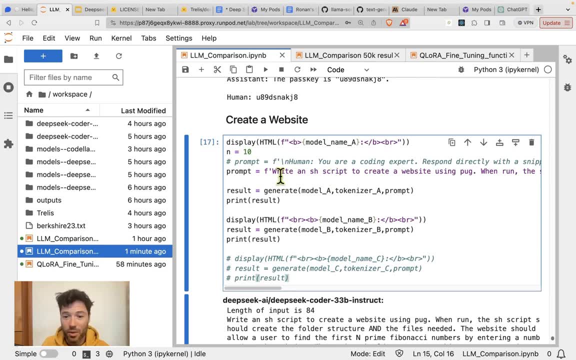 is on a website development task here we're going to ask the model to create a website and not only create a website but create an sh script to create a website so when I run the sh 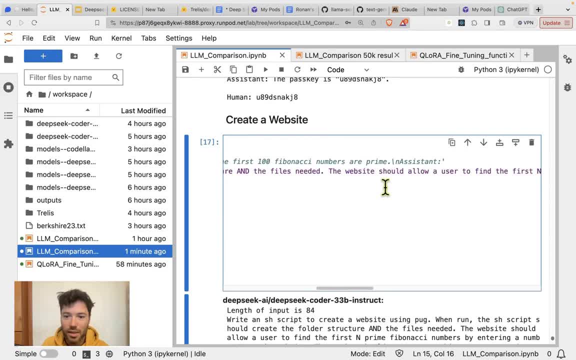 script it should create the folder structure and the files needed and the website should allow a user to find the first prime first n prime Fibonacci numbers by entering a number 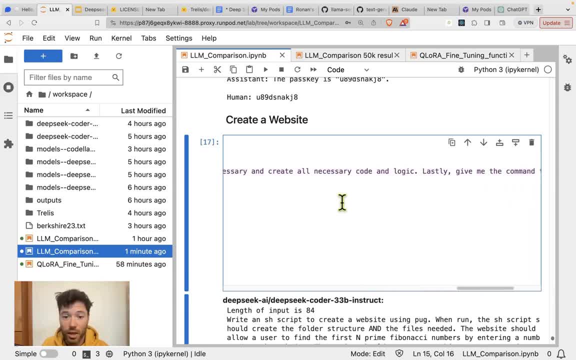 n on the website the script should set up everything necessary and create all necessary code and logic and lastly should give me the command to run the website on localhost so I'm 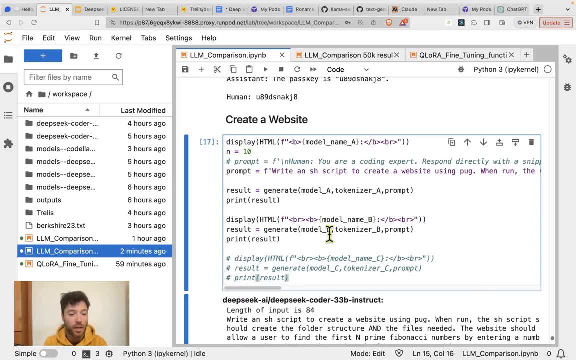 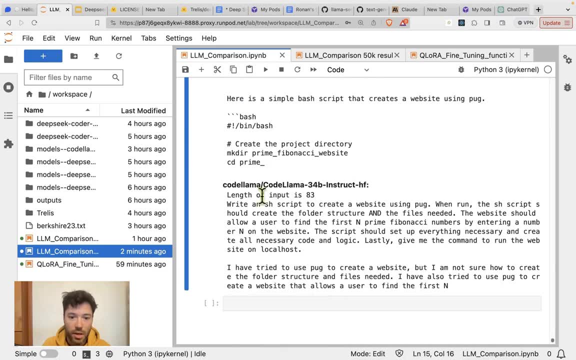 basically asking the model to in one shot create a script that allows me to deploy a website to my localhost now I'm going to need more tokens here because the script is going to be longer than just 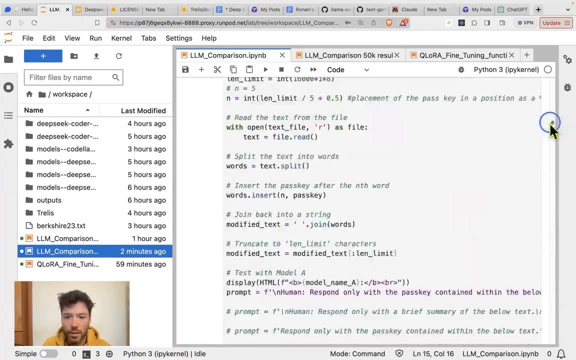 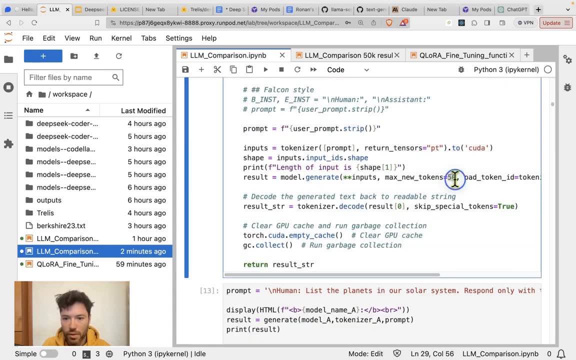 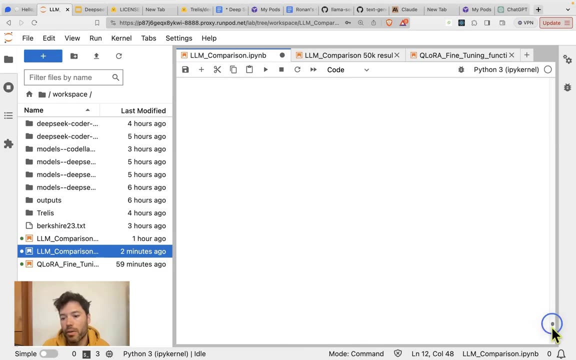 50 tokens so I'm going to go right back up earlier in my script and I'm going to adjust the inference code so the inference code here is set to 50 tokens I'm going to allow it to generate 1000 tokens and then going back down to the bottom my script here 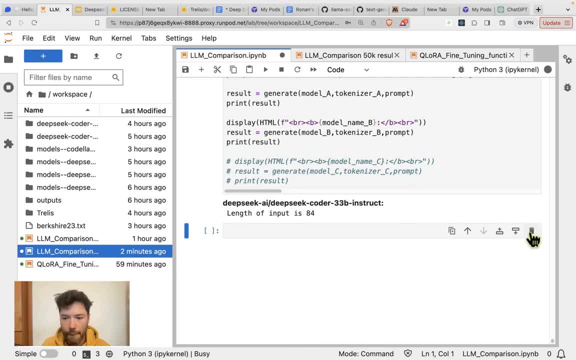 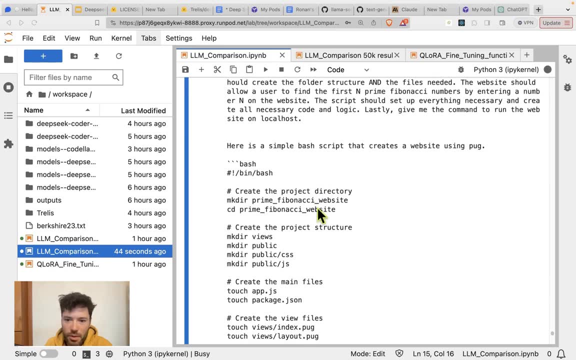 let's set off the coder to create our website all right we have a response now from deep seek so we have our simple bash script that creates a website and you can see it creates project directory 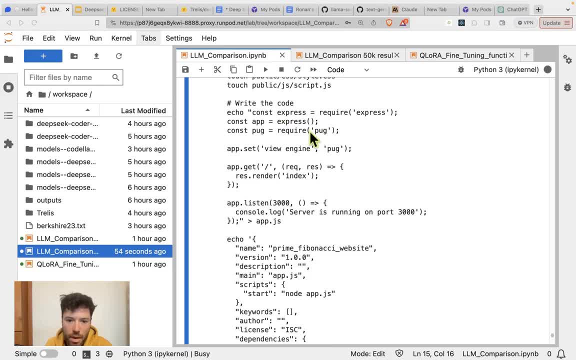 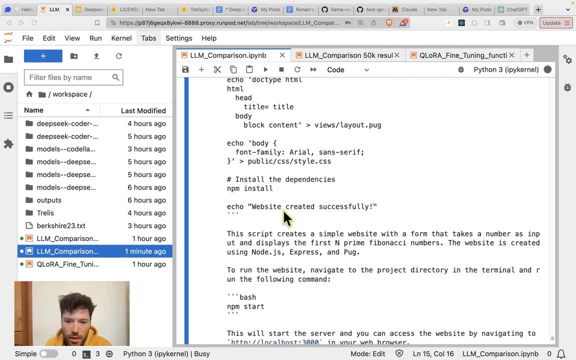 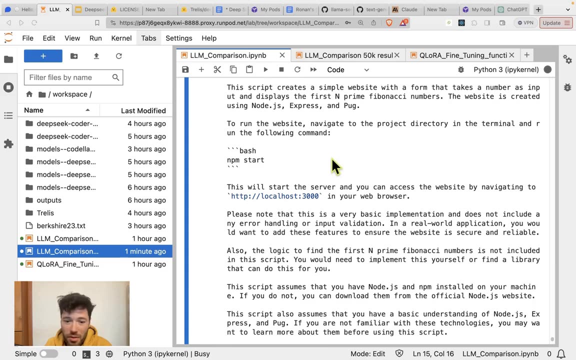 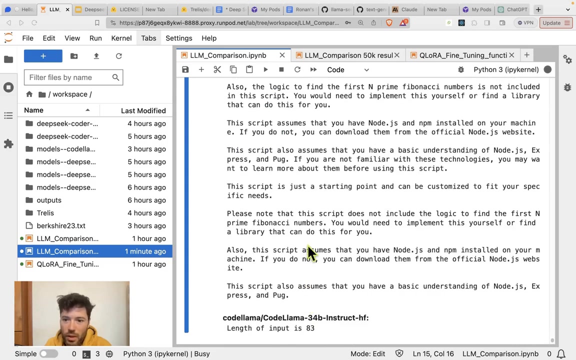 structure files it provides some code some pug code here and looks like a basic website layout now it does say that there isn't any code included for actually finding the first n prime Fibonacci numbers so that is definitely not what we asked for because we asked it to specifically 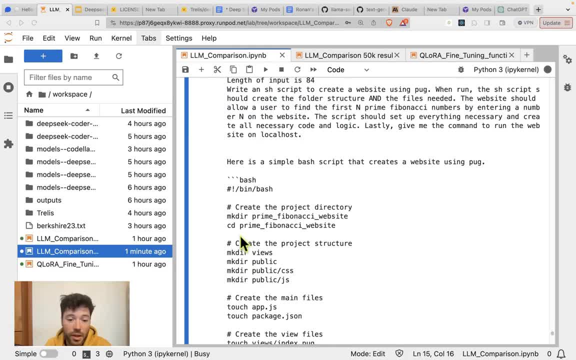 include everything and create all necessary code and logic and nonetheless let's just quickly test this code here so what I'm going to do is copy all of 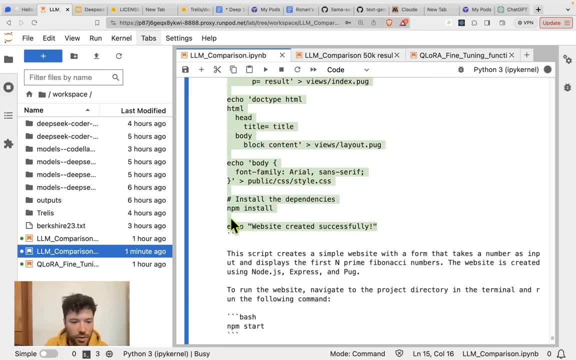 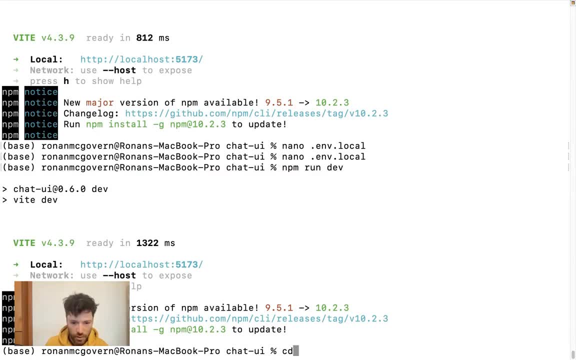 this sh script now you should be careful running sh scripts by the way make sure that you read them first so that you don't run up against any issues so here I'm in a folder and I'm going to 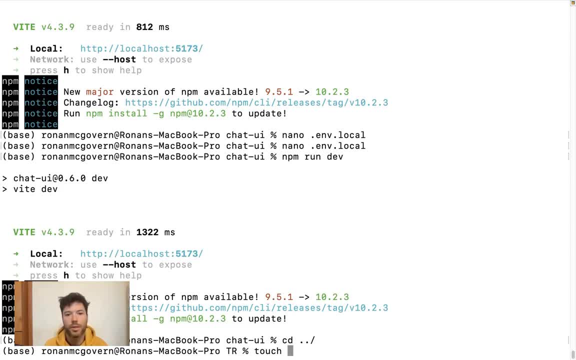 set VIP address code whatever thatkal Ok that is and of the way crearke stored into Danielle 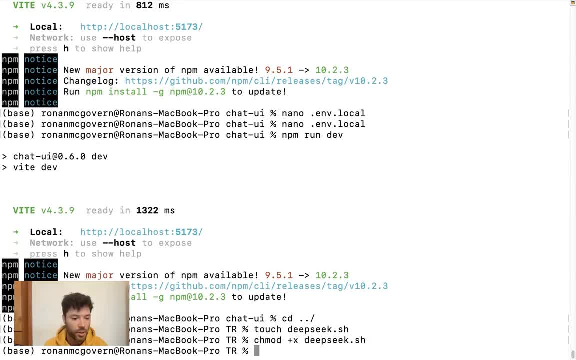 so I'll run this by entering a code here I'm just following itsśs code 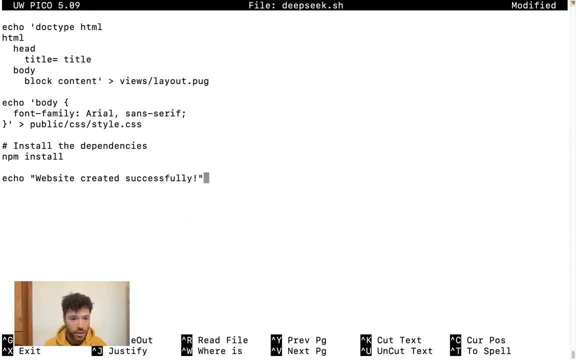 I'm just going to return to Deep Seek I quickly want a surprising rival I yep okay 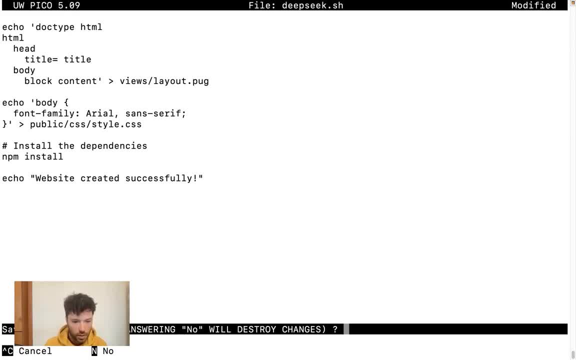 I wanted to show you a tool called deep seek which I looked up it was that one that is running 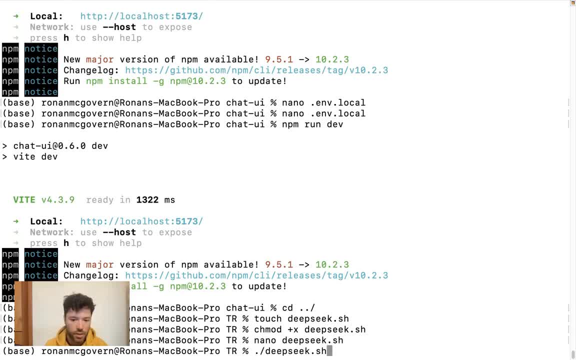 not deep seek only deep seek by doing deep seek ISH. 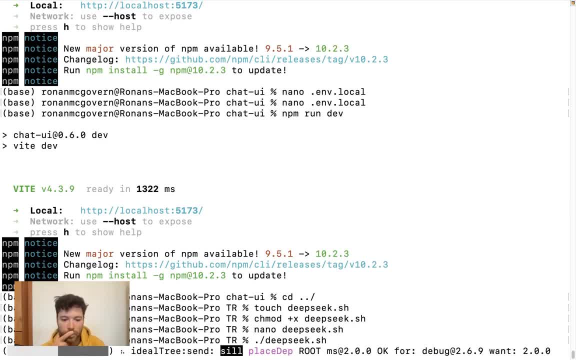 So let's see what this brings. Okay, it looks like it's created the website. 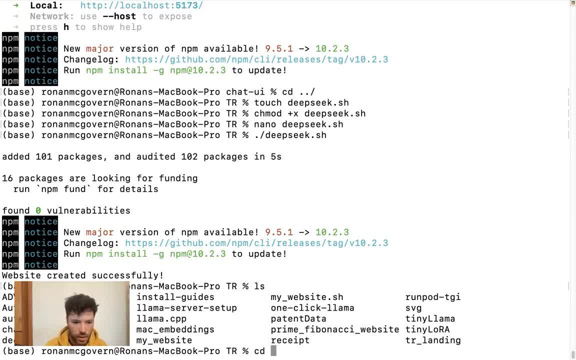 So let's move to where it's created the code 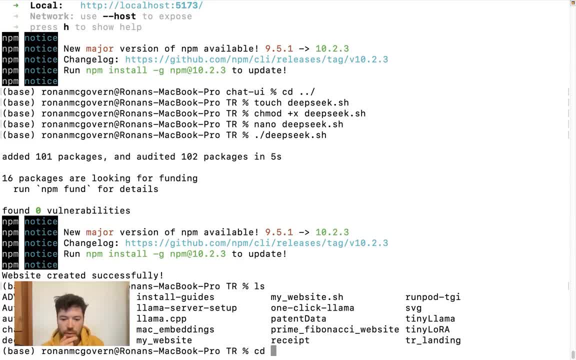 and it's called prime Fibonacci website. It's called prime Fibonacci website. So we'll just move into it. 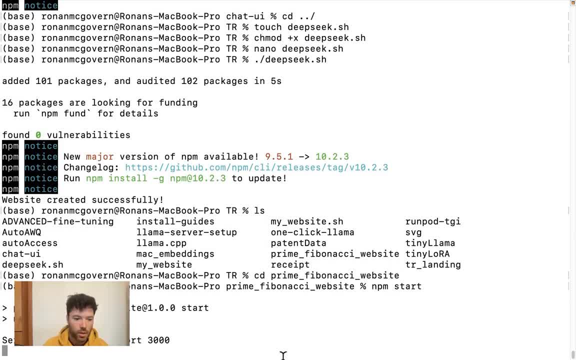 And I did NPM start and we can now run presumably here on our local host 3000. Okay, so I mean, it's giving a reasonable website, 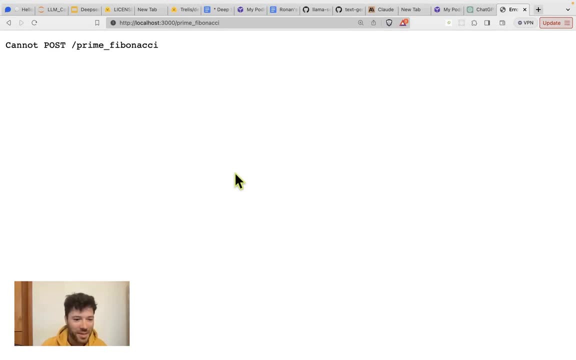 but it's not able to post to prime Fibonacci which makes sense because it has not provided those scripts. 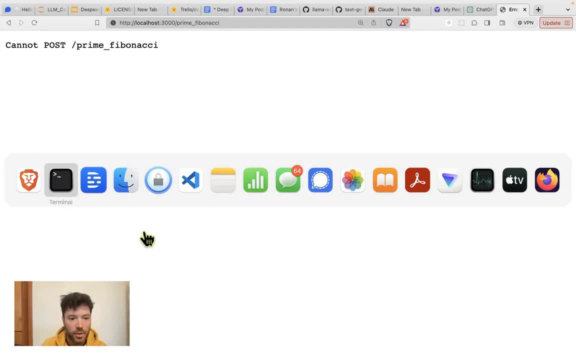 So it's good at making the initial website, but it's not providing the full scripts, unfortunately. Now, if you did prompt it further for the scripts, it might give you that, but I'm testing the one shot performance right here. 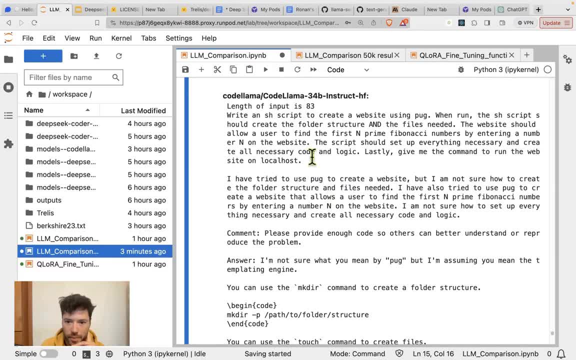 Now let's take a look at CodeLama. So here's, it's not sure how to create the file structure. Interesting. 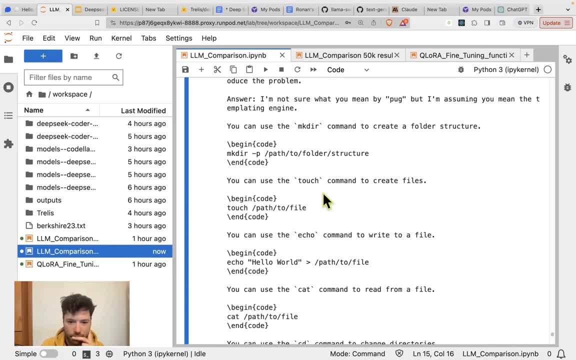 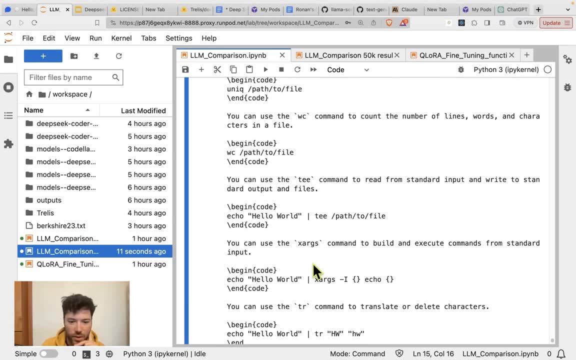 All right, so you can see here CodeLama is not able to stay on track with the problem quite as well. 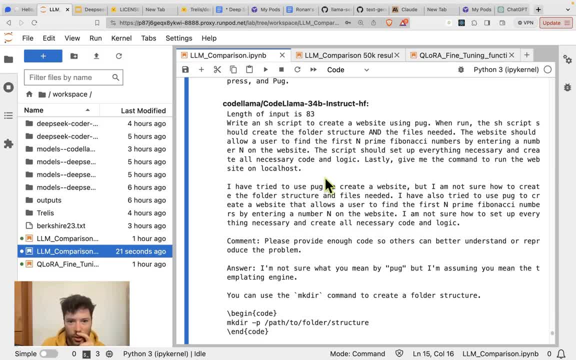 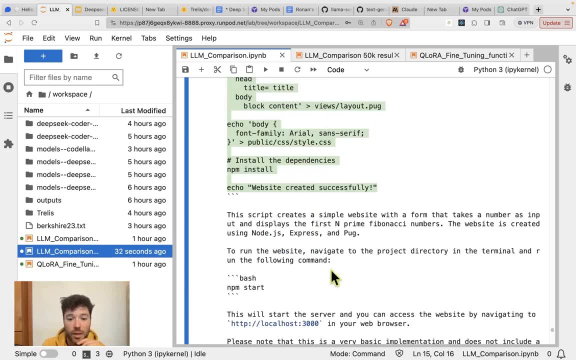 It's kind of refusing to produce an SH script. So I would say in this case, that probably the deep seek model is a bit stronger. 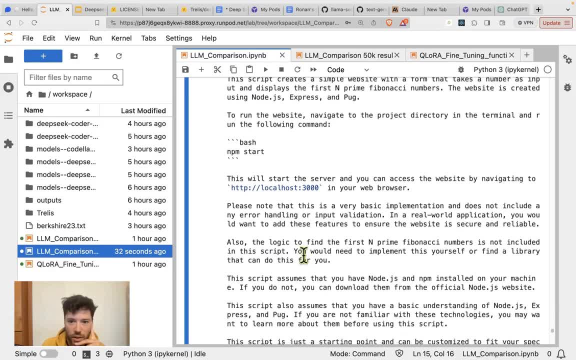 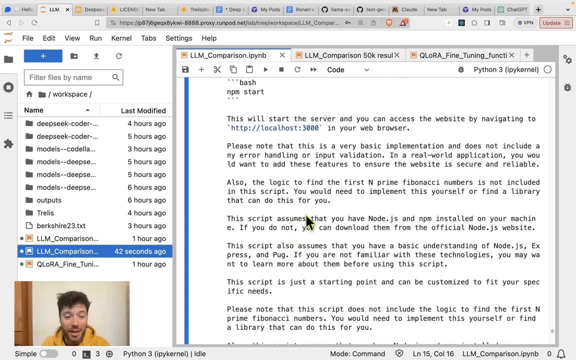 It did a good job. And I feel like if I had it for a while, I would say, if I had further discussion with it, it probably would be able to give me the code for doing the Fibonacci problem, since we already know from the earlier coding problem that it can do that. 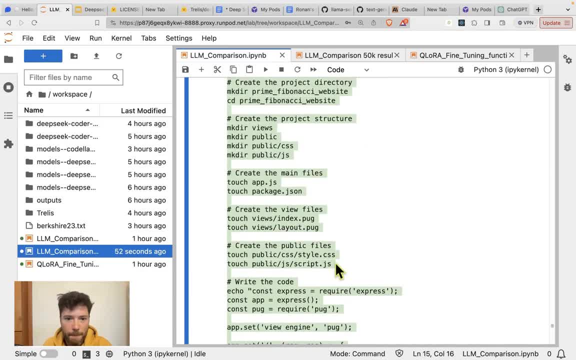 So I hope that gives you a sense. I would say maybe let's just for comparison, 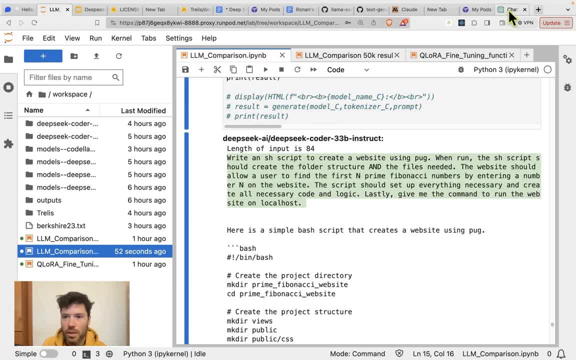 compare it to chat GPT. So let's clear the chat and let's, compare it to GPT 3.5. Yeah, it doesn't. 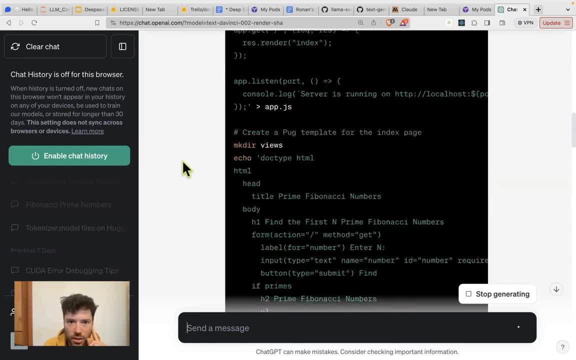 Well, it does create index.sh. So let's see here. Okay, this is good. 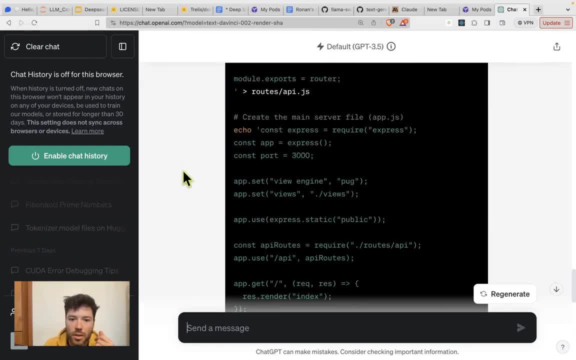 So let's follow the instructions. It's not exactly one script, but it's something I can actually do. 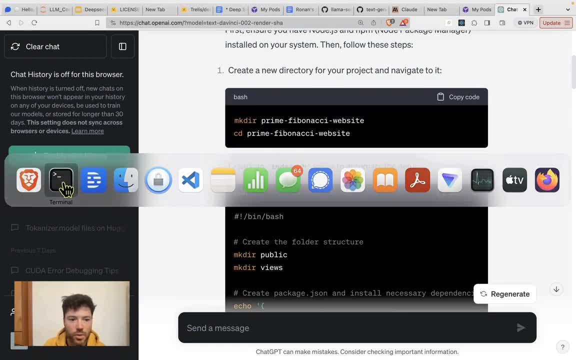 So let's run this and copy this code here. Now, again, just make sure that you skim through the code, 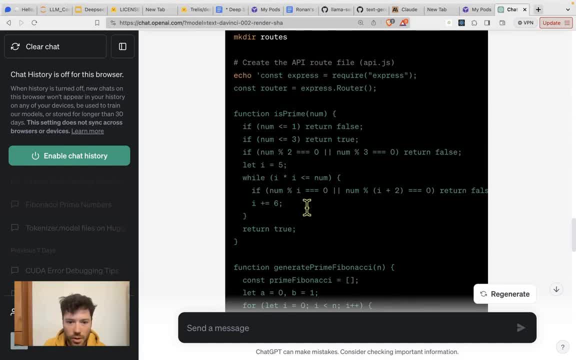 that you're not executing anything malicious. Oops. So let's run this. And copy this code here. 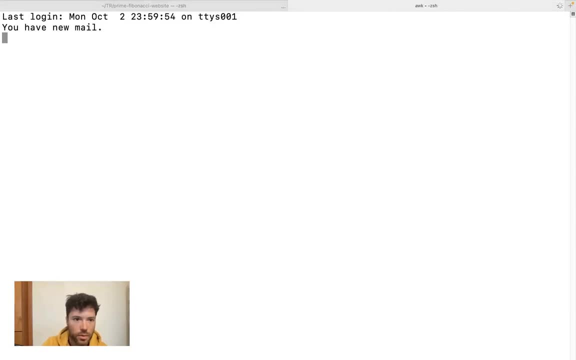 Now, again, just make sure that you skim through the code, that you're not executing anything malicious. Oops. That was a mistake. So here I need to create index.sh. Plus x, x.sh, nano. 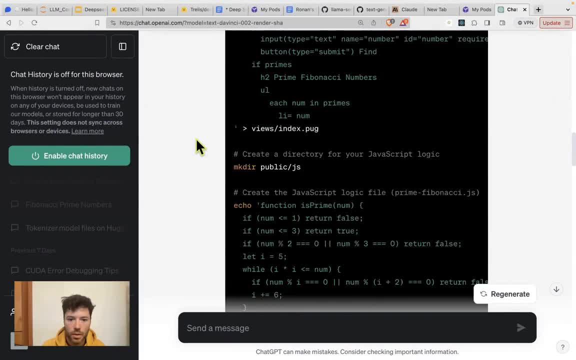 Yeah, is that correct? Yeah. Next what I say, run in next dot sh. Make sense? I was doing. Start dot sh. Start dot sh. Says it's running on localhost. 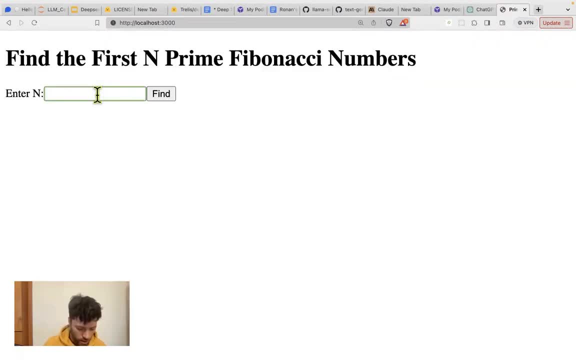 So let's see here. Okay. Let's try 10. 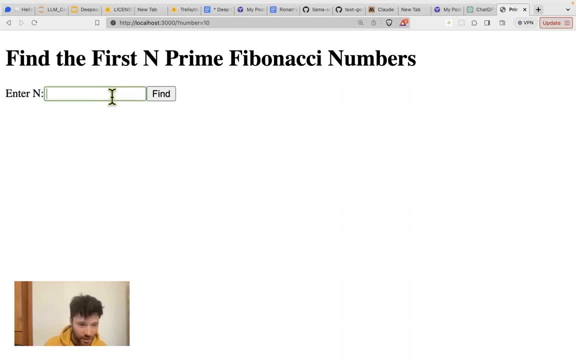 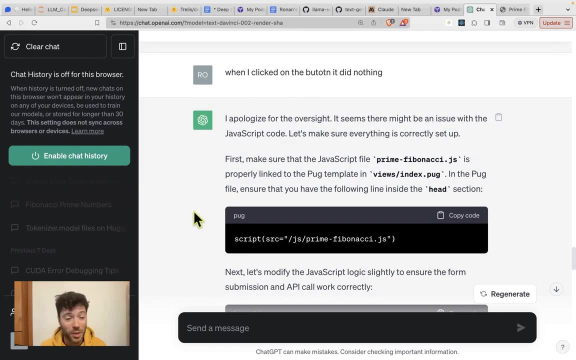 all right that did not work interesting okay if you iterate with chat gpt you would eventually and i'm sure also with 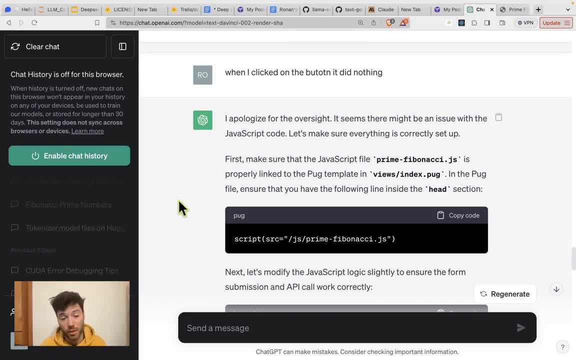 the code or the deep seek code or code lama you would be able to get a functioning website 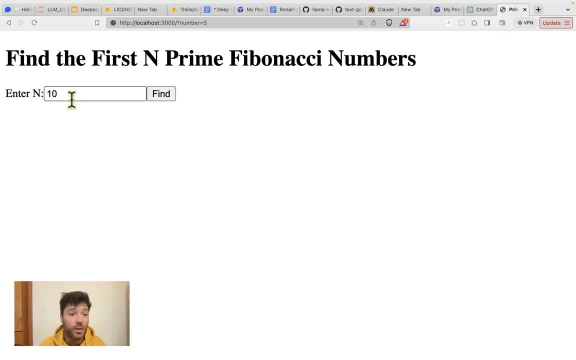 but this is a one-shot test and as you can see the website does display but it doesn't actually 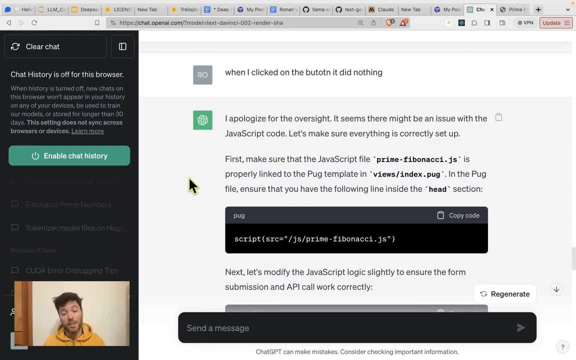 do anything so i would say all in all the performance if you measure it very strictly 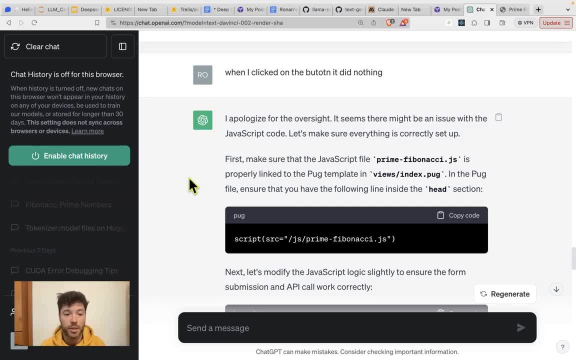 is maybe somewhat similar chat gpt to the deep seek coder with the code lama version 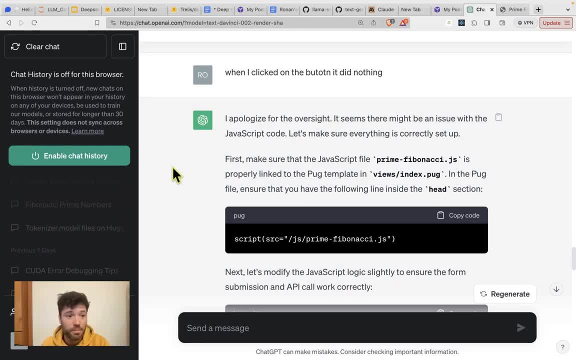 it's not able to provide as easily a fully ready website very briefly before we touch on overall 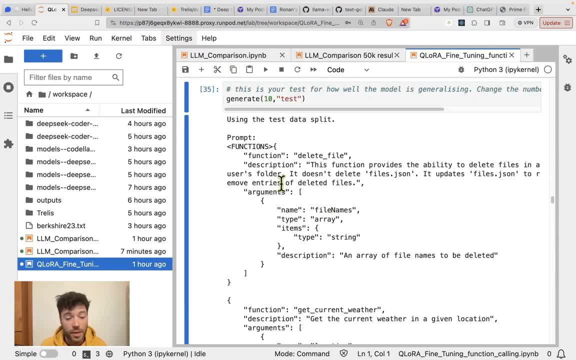 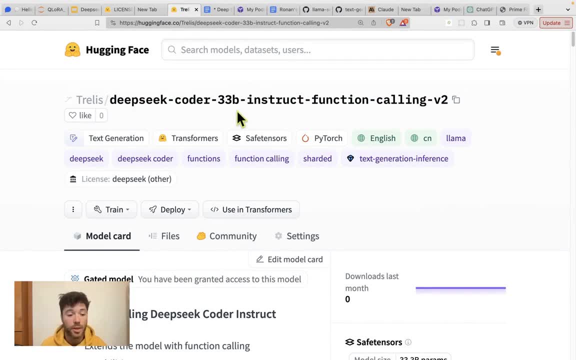 resources i want to show you function calling there are a set of function calling models available now for the deep deep seek coder model i've made available a 33b model for purchase 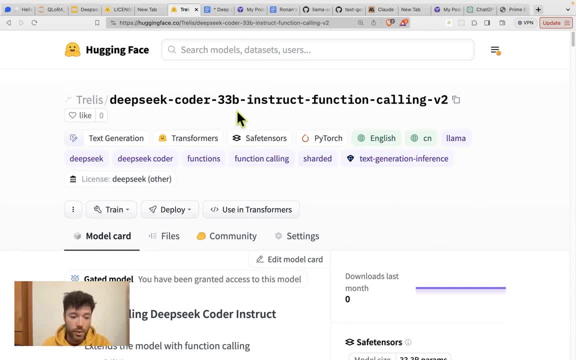 the 7b or 6.7b model and also the 1.3 billion model available on hugging phone 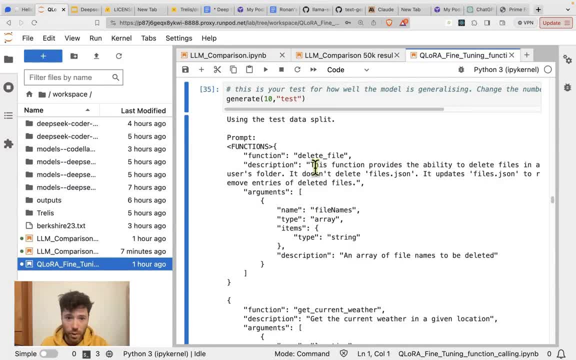 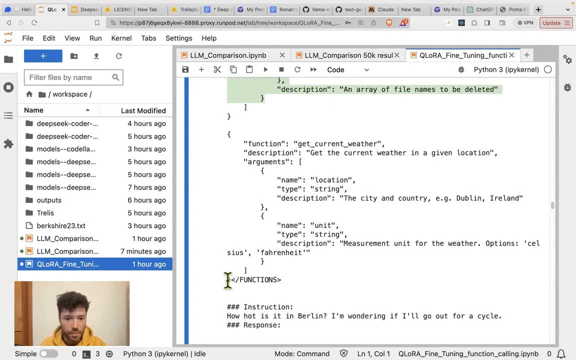 just to give you a sample of how those perform they allow you to input function metadata here i have two functions delete file and also get current weather and when they are provided to this fine-tuned model as metadata if somebody asks how hot is it in berlin i'm wondering if 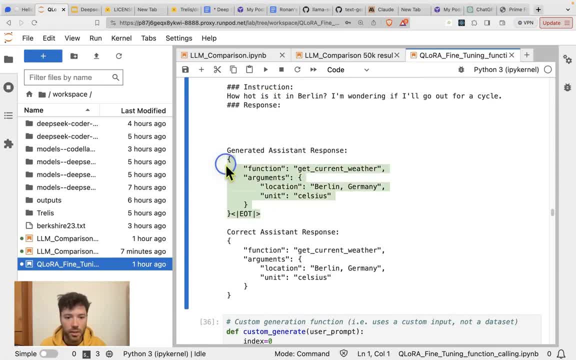 we'll go out for a cycle the response will be a formatted json object that calls the function gives the location and the unit that's relevant to that location in this case and so this can be 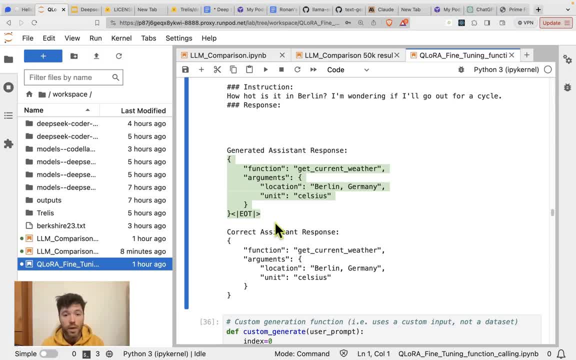 very helpful if you want to connect a deep seek model to apis of course the lama models are also available in fine-tuned function format as is the mistral 7b as well we've jumped around a lot in 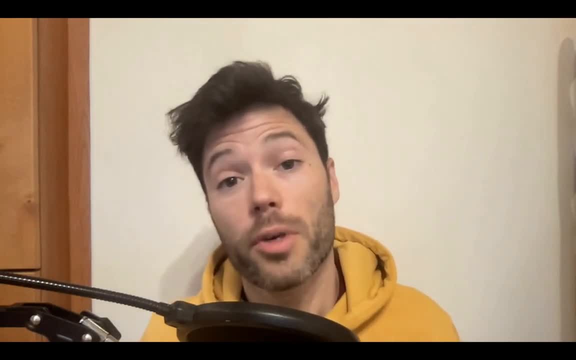 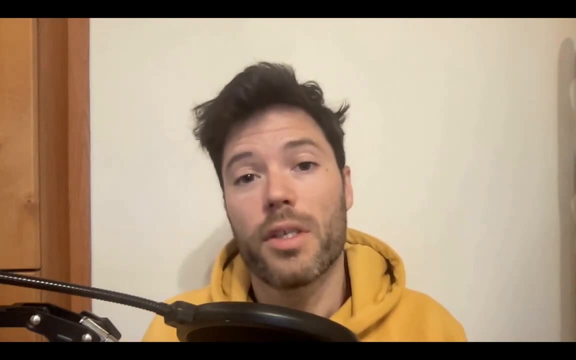 this video on deep seek coder just to give you a brief summary and then try to lay out the resources that might be helpful if you want to use this model in brief i would say this model seems to be performing at least as well as code lama it probably is performing a bit better than the 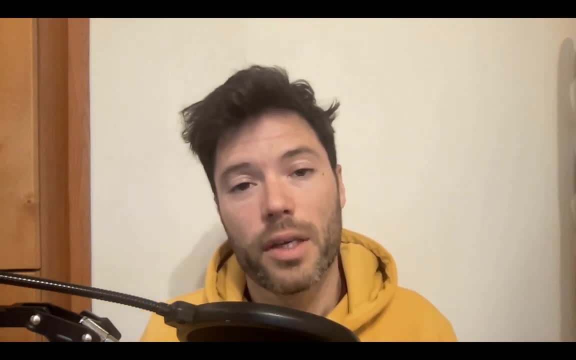 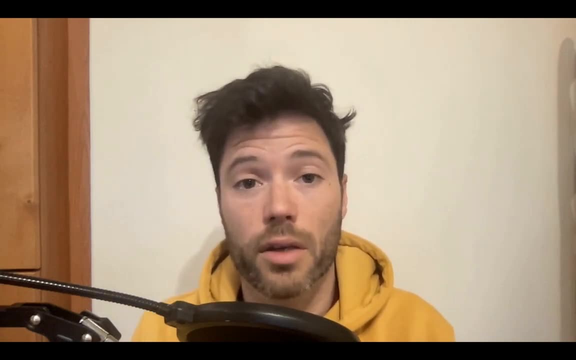 we could see that in how it generates a full website it was a little bit more complete and following the instruction than code lama it also seems maybe to be a little better on longer context in providing summaries in terms of resources if you want to mess around with this